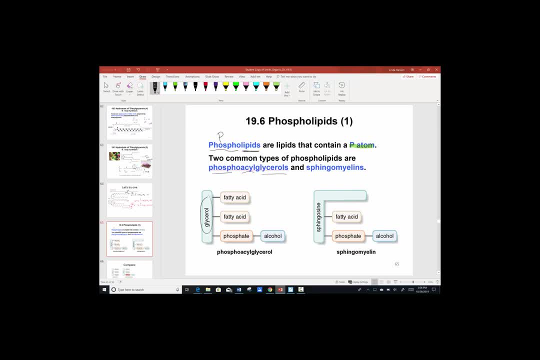 backbone out again to play. And then a little different molecule called a sphingomyelin and, I think, always a neuron, especially like a neuron sheath for myelin, Our general structure for a phosphoacylglycerol. again, we're going to just take a quick peek. 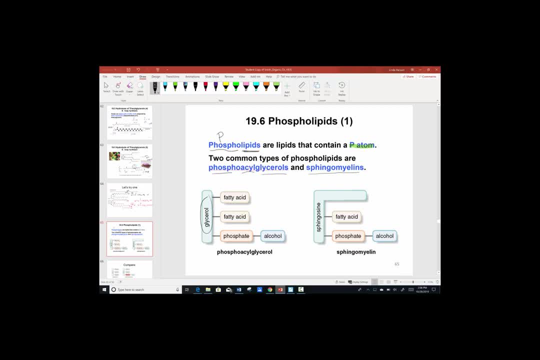 at drawing these general structures. We're going to put a kind of a vertical glycerol molecule straight up and down, but we know specifically by now that a glycerol is a three carbon chain and what we'll see here is an ester linkage. Two of the three bonds two: 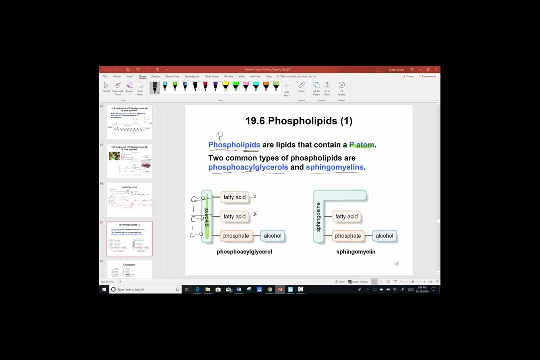 of these three bonds are identical to triacylglycerols. they contain fatty acids from our section two, that very chart that I gave you in the front of your note pack page. But what makes them unique is this third attachment, which we see: a phosphate, If you remember a phosphate. 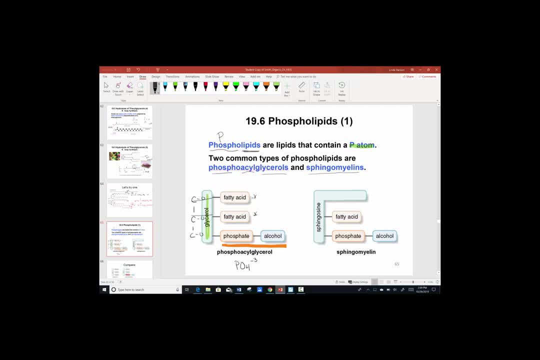 from inorganic phosphate is a polyatomic ion that has a central phosphorus and four oxygens going around in all directions. There's a formal charge on the phosphorus of A minus three and actually we'll start to see that there'll be some double bonds leading to those. 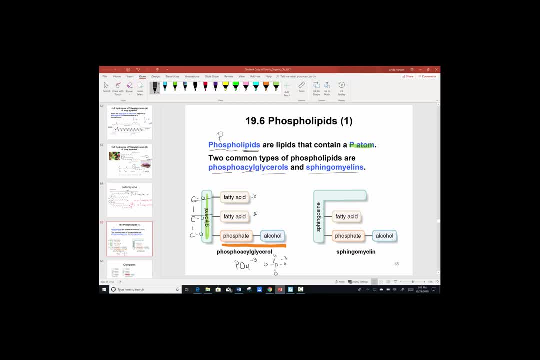 oxygens, And then that phosphate is leading out to an alcohol, an OH group. So what makes a phosphoacylglycerol molecule different from the fatty acids we were studying before is this third attachment involving the phosphate linkage. So let's compare that to a sphingomyelin and we see that no longer do we have glycerol. 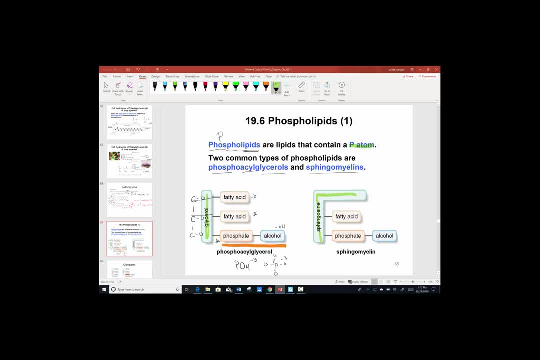 as the backbone, but we have a separate kind of a different backbone. There's some similarities when we look at it's carbon structure, but a sphingomyelin replaces glycerol and puts sphingosene into its place. We still have one fatty acid and then notice this is the 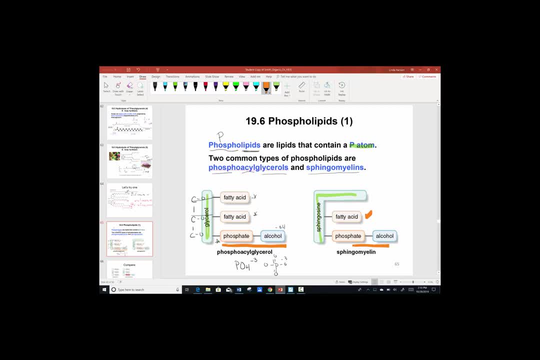 same, a phosphate-alcohol glycerol, But its water-based. So the second appearance is a phosphoacylglycerol to the body acid. So we see it's there is a phosphoacylglycerol to the group. So one of the fatty acids has been replaced as terms of the tail part of the 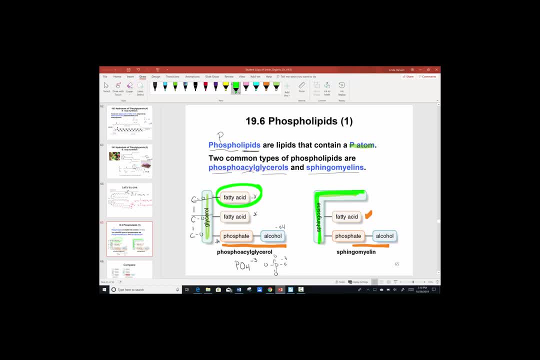 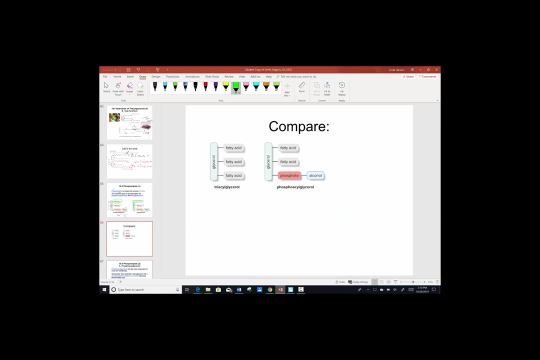 actual structural backbone, leaving just one fatty acid to attach and again identical phosphate alcohol in that third bonding position. So if we compare a triacylglycerol from what we were just drawing to a phospho-a-glycerol molecule, we can see that the difference is. 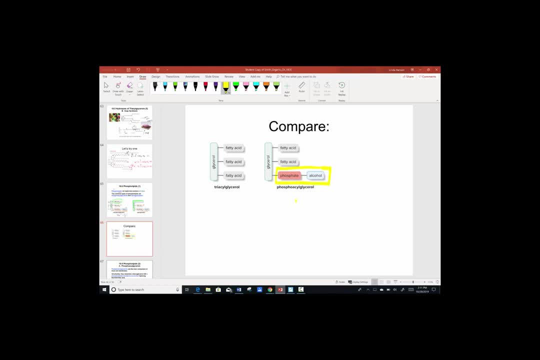 in this third attachment, where we have a phosphate, a PO4,- that's a marker- we have a phosphate, PO4-3, giving us that structural phosphorus grouped here, phosphorus in the central region and of course, leading out to an alcohol, And we'll develop some of those very 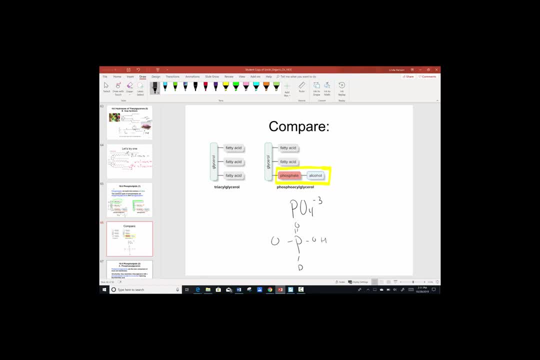 specific structures. but just comparing triacylglycerols to a phospho-a-glycerol, it's that third attachment that makes them different. They are the major component of most cell membranes and that's probably where we've heard them most often. A phospho-a-glycerol are the main. 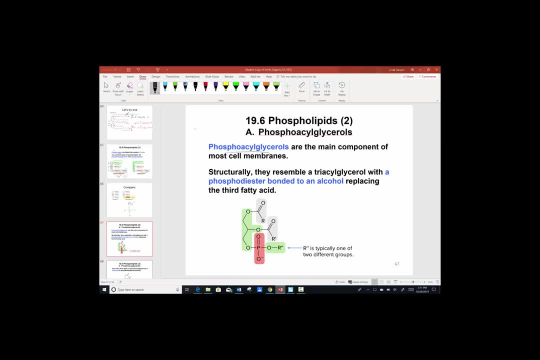 components of most cell membranes. So structurally they do resemble the tri-a-glycerol, which is known as the triставля, which means liquid怎 Surprise her? but instead this has prepared something else. Now, whenever we look in the brain, there's an element of phosphogylaminin. 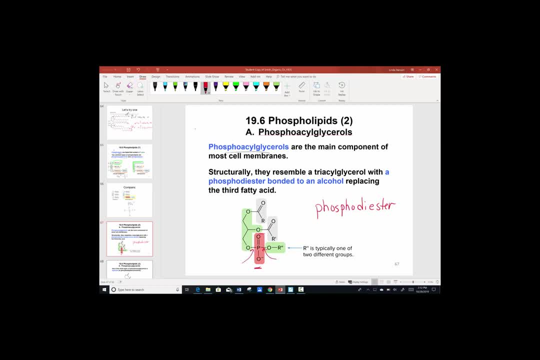 siguiente, again swimming up and down. So this polymer has a hugeallo going in. so instead of just going up, we have a polysaccharide here and into allowable insertion there's photogénesis. okay, Now why is photogénester toxic? in the team, It turns out this is a всё fragrance and there's new obstructions to alcohol. mudar the Glycerol bonding. 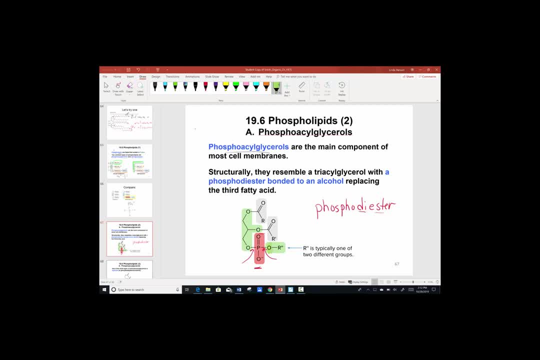 ester linkages, and there are indeed two ester linkages, but the linkage attaches to a phosphorus instead of a carbon, as it would in a fatty acid. One of the main types of phospho-aglycerols, phosphoacylglycerols, is cephalin or it. 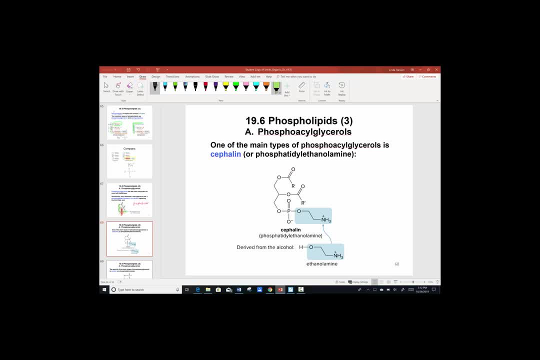 gives us a long name based on its chemical structure. We see the root word phosph. atidi ethylene-ol for the alcohol and amine for the nitrogen. We'll call it cephalin. When I look at this particular structure, I can see that this: 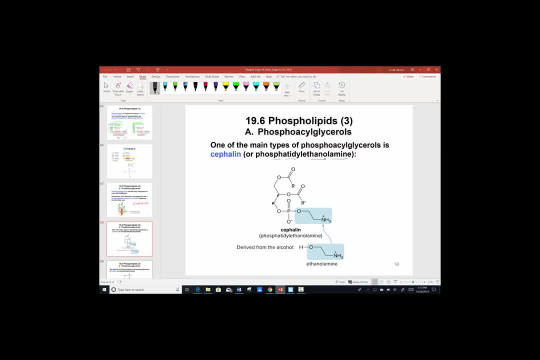 is a phosphoacylglycerol, so we have the glycerol backbone. There's the original glycerol, that was the three carbon chain. Glycerol has those three alcohol units In place in. I'll call this position one. we have an ester linkage leading to a fatty acid And in position 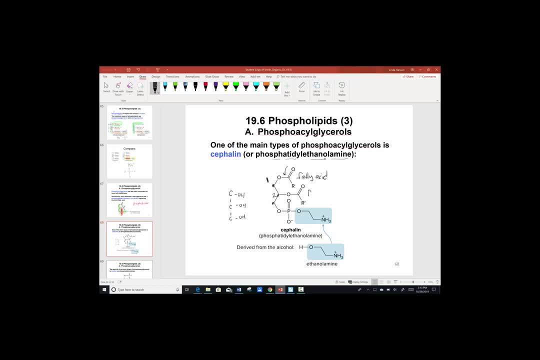 two, we still have that ester linkage leading to a fatty acid. And now, in cephalin, here is the new portion compared to the triacylglycerol backbone. And in position three we have the phosphoacylglycerol from before Carbon. 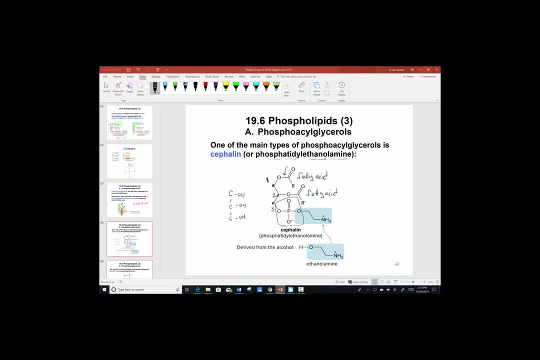 number three leads to a phosphate, a PO4 unit, And so the phosphorus, leading up to a double-bonded oxygen. Two of the oxygens are bonded in a linkage, And the negative charge on this oxygen is critically important because it's there. 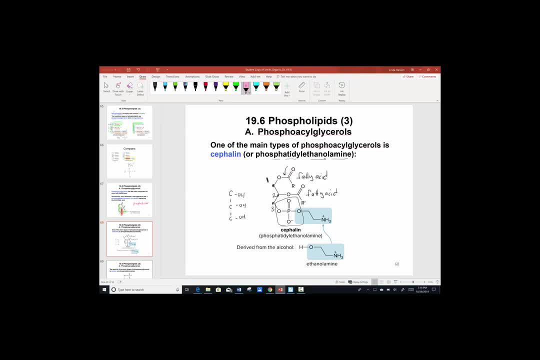 to electrically balance the positive charge on the amine group. So emphasize, okay, You know that you have to activated a negative charge on the oxygen and we're balancing that negative with a positive formal charge on the amine group. So here we have a new. 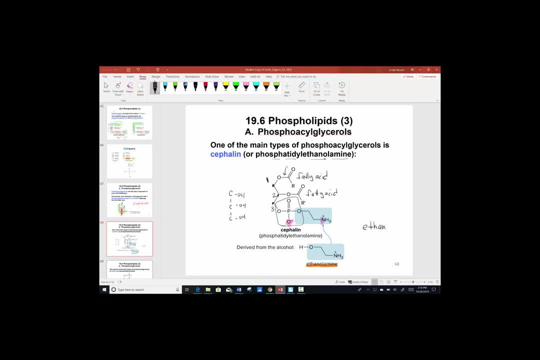 word ethane-ol-amine. Ethane-ol-amine, The ethane-ol is a two-carbon alcohol group, Carbon one, carbon two, A two-carbon alcohol group. The term amine is the nitrogen, and we just finished a chapter devoted to the amine chemistry. 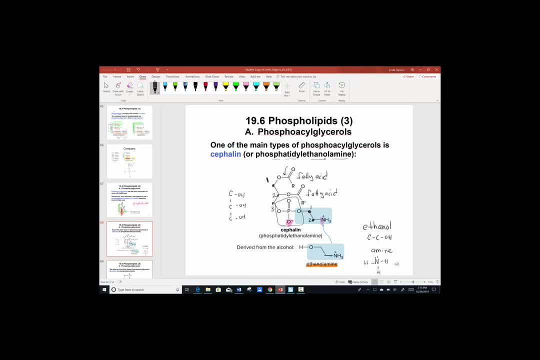 And notice based on formal charges. it has an attachment. it's four bonded, so we can think of that as four bonds and we would have a plus sign there. So in ethane-ol- that's the alcohol part- amine is based in nitrogen, so it's just a. 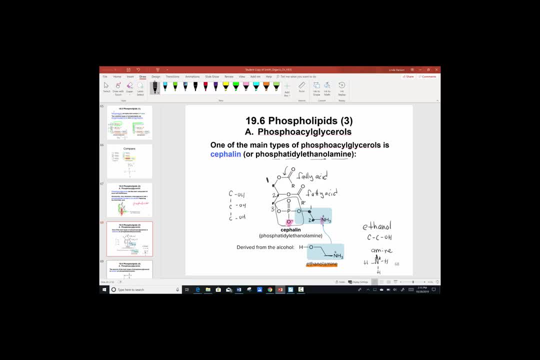 derivative of that alcohol portion, So cephalin. in that third position we have a phosphate ether linkage- sorry, there's the two ether linkage- and then it leads to a two-carbon ethane-ol amine group. Another type of phosphoacylglycerol is called lecithin, lecithin, and again it also has. 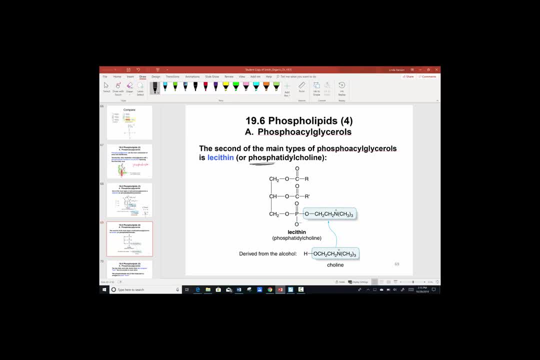 a long chemical name based on what its structure is, A phosphoacylglycerol, Phosphatidy, and then again notice we have the phosphate group and then we see this part here saying it's atidal choline. choline is this part of our molecule from the alcohol. 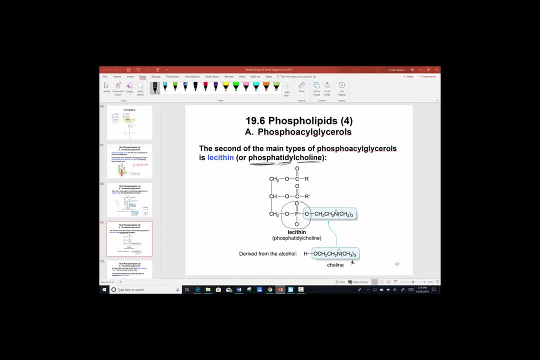 We're stressing, a lecithin product will have the phosphate and instead of a monosubstituted nitrogen we have a trisubstituted nitrogen. all with methyl groups And it's a four-attachment. I'm going to go back a slide to emphasize. 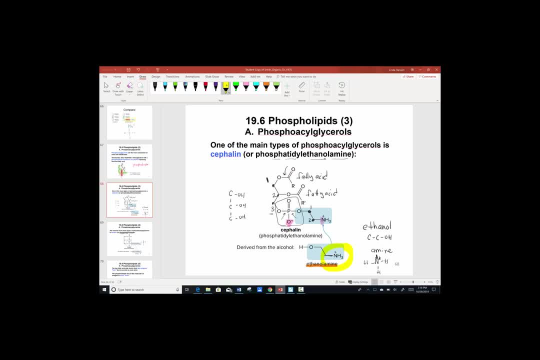 Notice here, the nitrogen all led to hydrogens. It was simply a monosubstituted amine where the nitrogen attached directly to the alcohol In our next type of phosphoacylglycerol. in this last portion we have a trisubstituted. 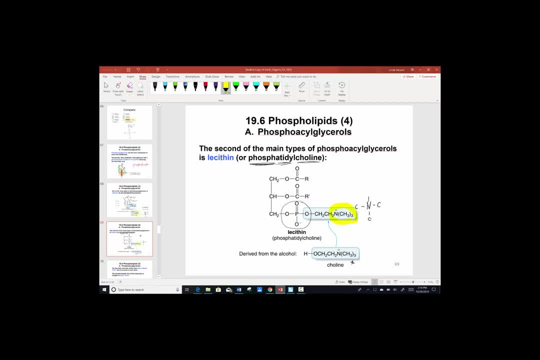 nitrogen in which all directions lead to a lecithin. So we're stressing a lecithin, lecithin, and again it's a four-attachment. I'm going to go back a slide to emphasize. Notice here: the nitrogen all led to hydrogens. 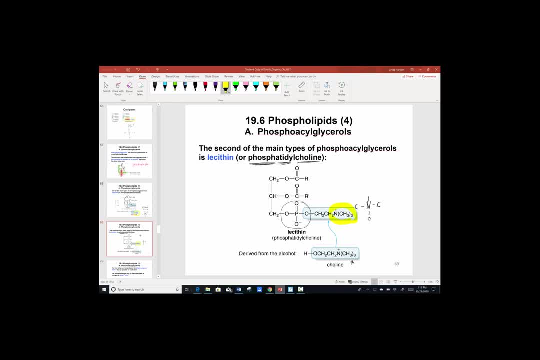 It was simply a monosubstituted nitrogen头, led to a lecithin and again it's a four-attachment L. Spain. lasithin is a second main type of a phosphoacylglycerol. These two fatty acid genes are very nonpolar tails and they lied parallel to each other. 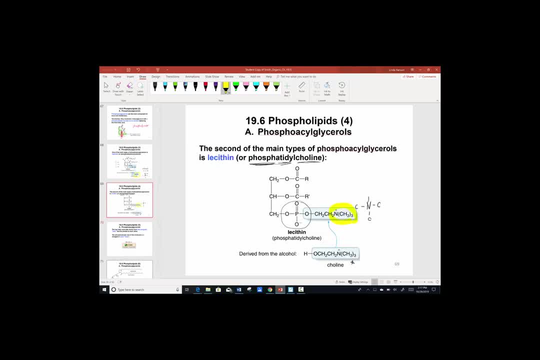 And that phosphodiester end of the molecule is charged with the polar head. I'm going to back back up and say This region, but we have these very long fatty acids. those long fatty acids are a non-polar chain. They are what we refer to as hydrophobic water hating. 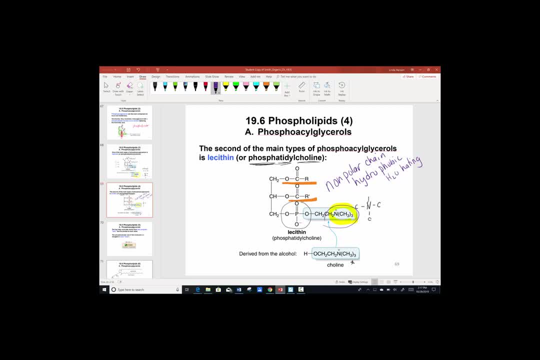 But here we have a very charged area. We see that that oxygen is carrying a negative charge, The nitrogen is carrying a positive charge And that creates what we have as a polar region of the molecule. And because it's polar, it is said to be hydrophilic: water loving. 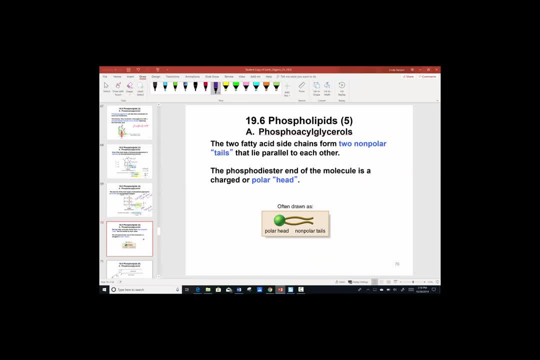 And that general structure there has a polar head, which is the charged positive and negative region of that phosphodiester. And those two tails represent those two fatty acid chains, those long carbon chains that were hydrophobic. Water loving is the phosphodiester region, polar head. 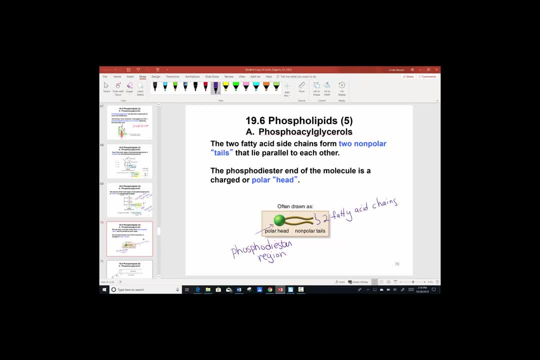 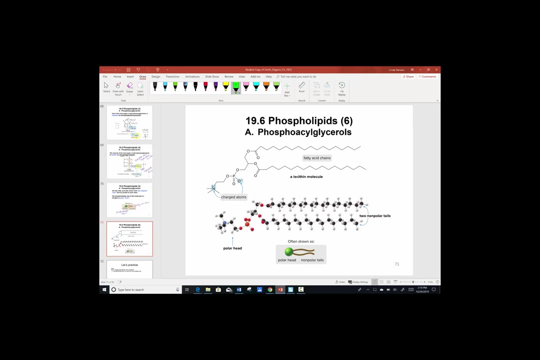 Water hating is the fatty acid chains, the non-polar tails, Very important structure really in the structure of a membrane, as we'll soon see. So here we have a molecule, a phosphoacylglycerol, And we can see that it's a very complex structure, but I can see some similarities. 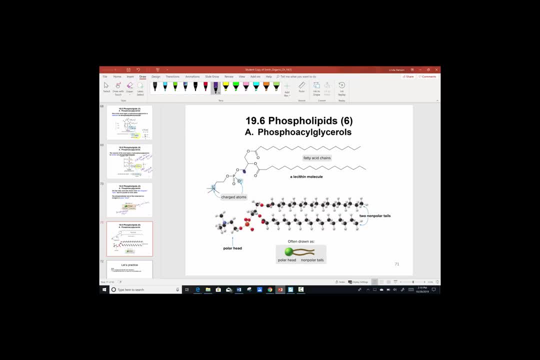 Notice here right off the bat I want to point out: here's carbon one, carbon two, carbon three of the glycerol backbone. Okay, Okay, So I can still see the same backbone as the glycerol molecule, And in position number one- I'll call this position one- I have a long carbon fatty acid. 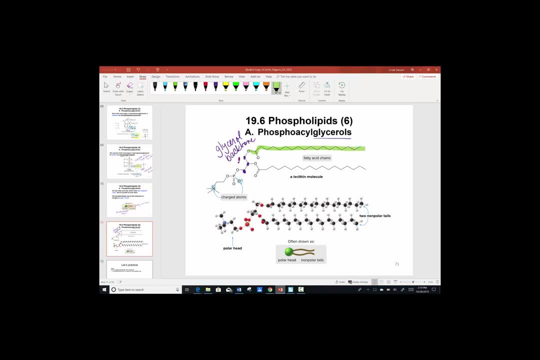 chain. I also have that in position two, So when I label this as carbon two, I can see a second long carbon fatty acid chain. These are referred to as the tails And they are hydrophobic water hating because they are indeed long carbon chains, non-polar. 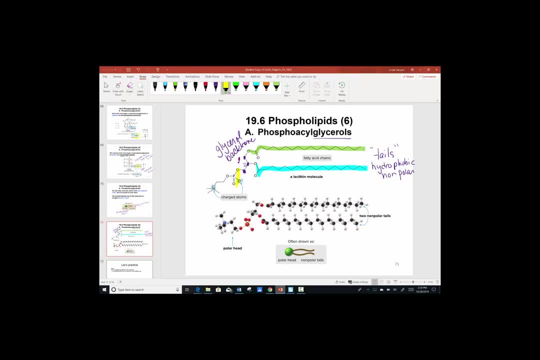 Down here I can begin to see the phosphate group. Remember these phospholipid bilayers. phosphoacylglycerols contain a phosphate attached to the nitrogen And that nitrogen are very charged particles. We have a negatively charged oxygen here, balancing the positive charge on the nitrogen. 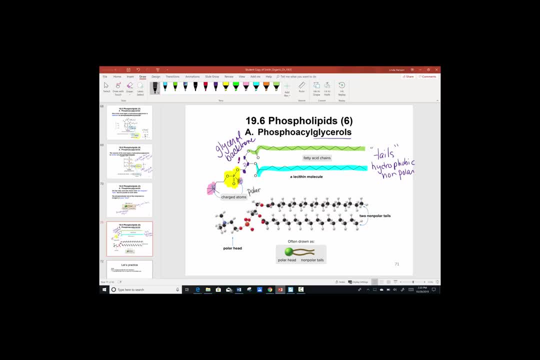 And this creates what we have as a polar region. We call this the head of the molecule And it is indeed hydrophilic water loving To generally draw that structure. very quickly. you'll see just this type of picture where we have a polar head. 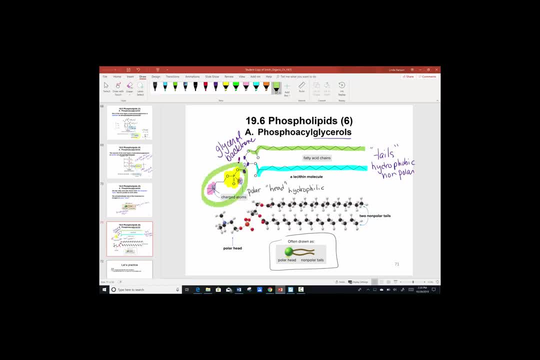 This polar head represents this region of the molecule. We have these non-polar tails. These non-polar tails represent these long carbon chains of the fatty acids. So polar heads and non-polar tails is a quick, dirty picture there. just a quick structural 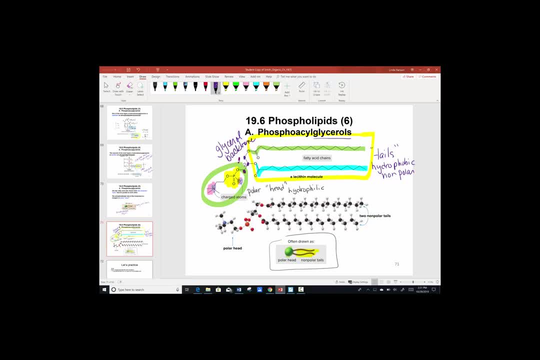 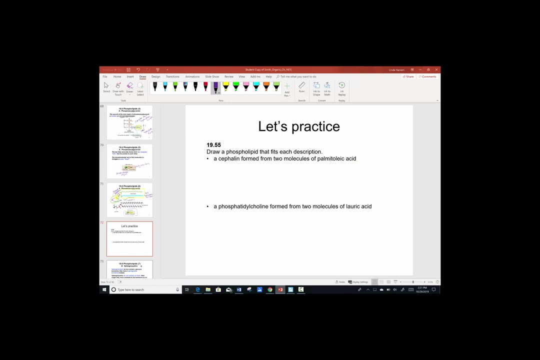 area to let us know that the head of a phosphoacylglycerol is very polar, coming from the phosphate group, and the tails are non-polar, coming from the fatty acid group. Well, let's practice Draw a phospholipid that fits each of the descriptions in the following. 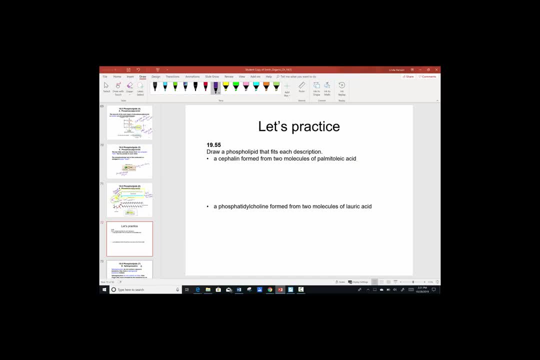 We want a cephalin formed from two molecules of palmitoleic acid. So I'm going to suggest you find your chart, because we're going to need to know palmitoleic acid, Excuse me, And then we can work to the next one. 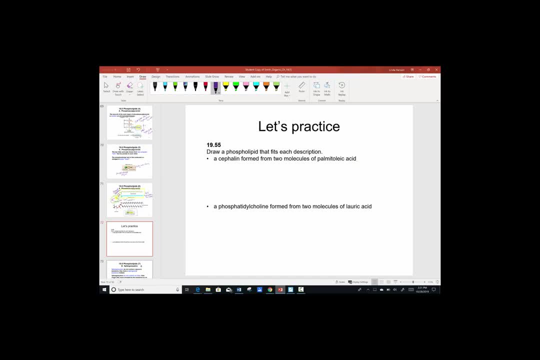 So find that and look up for me the formula of palmitoleic acid, and then just pause the video and come back once you've found it. Are you ready? Pausing the video helps, doesn't it? So welcome back. I know that you went to the trouble to find this particular fatty acid. 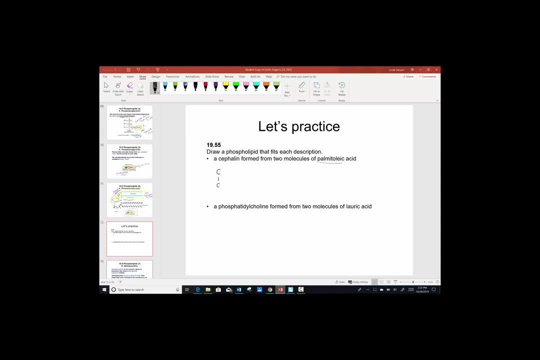 And so what we want to do is begin simply by drawing the glycerol backbone and knowing that the glycerol backbone still is going to contain the ester linkages The palmitic acid is. we just saw we can write this as CO and I'll just leave this. 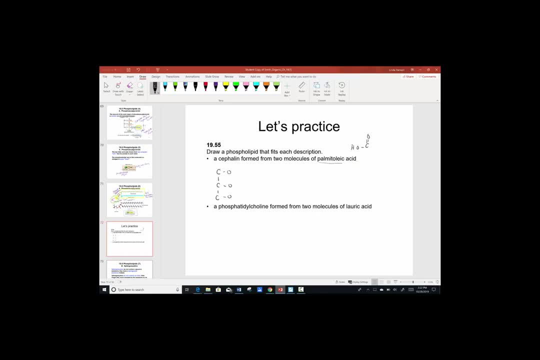 as OH. It will be in the acid form, even though we'll hook it as an ester linkage in a moment. We had CH2 taken seven times, We had a CH double bonded to the next CH, We had CH2 taken five more times and then finally, the methyl group, terminating the carbon. 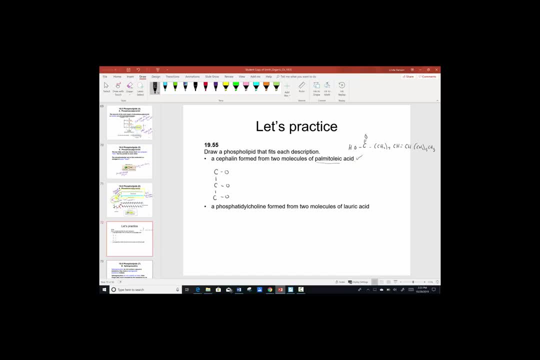 chain. So that's why I paused and let you do that hard work of finding that from your very front page of the note pack. It's a tool page. You don't have to know these by heart, But you do have to know how to find them. 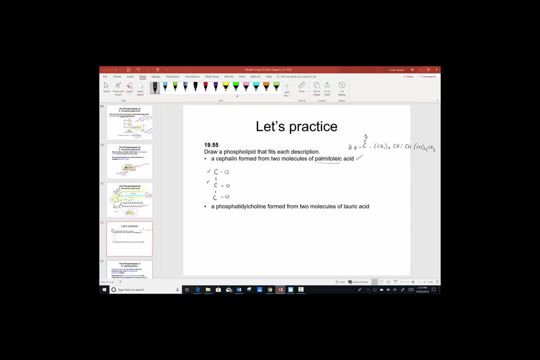 So I know that in the first two positions, first two carbons, they're going to attach to the fatty acid. So that's the general structure of our phospholipid. So I know that this particular O is going to create an ester linkage. and I'm just now. 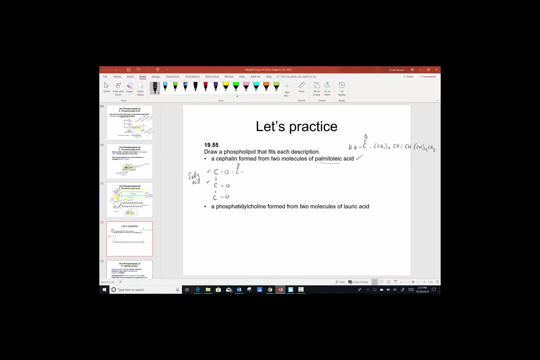 going to attach the rest of that fatty acid. So this is the carbon that I just drew here. I have a CH2 group taken seven times. Then I bump into that C, double bond C, Then I know that it's a cis conformation. 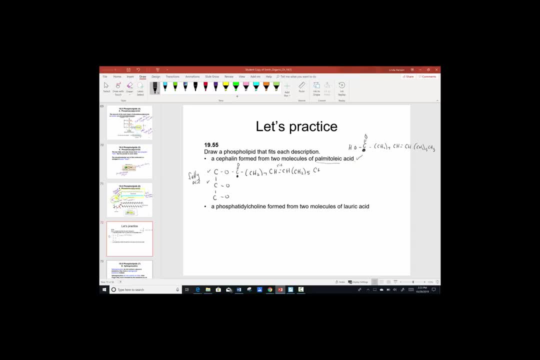 We have a unit of CH2 taken five more times and then, terminating with the alkyl methyl group, We have two identical fatty acids, So I just need to draw this twice. There we have it. So position one and two are indeed the positions of the two fatty acids we looked up. 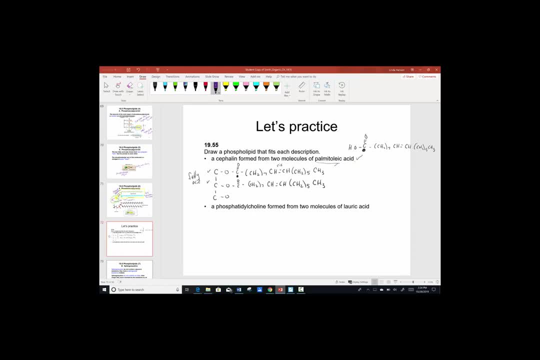 Palmitoleic acid, And then, of course, to make it a cephalin, we know that it now has a phosphodiester linkage, So the P replaces the carbon. And down below here I'm running out of room, so I'm just going to come to the bottom. 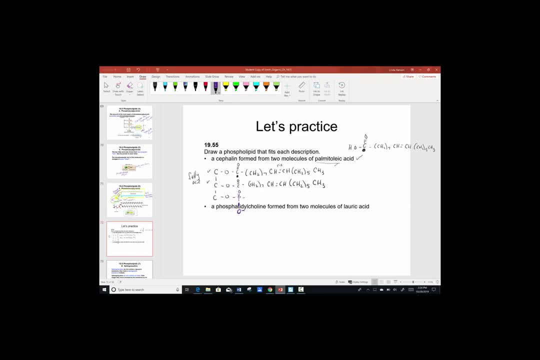 I know that that oxygen is charged with a negative charge. The oxygen pointing up is a double bond, just as it is above, except the oxygen now is attaching to phosphorus. We had a diester linkage. We made sure to place the bottom oxygen as a negative charge because we understand it's. 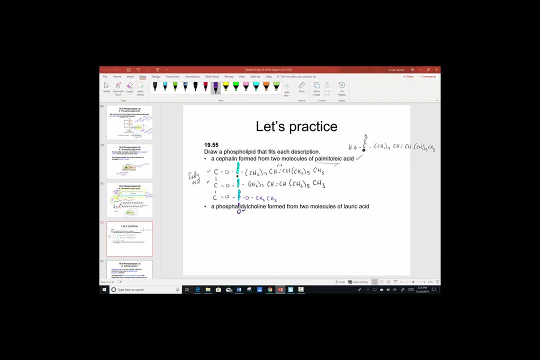 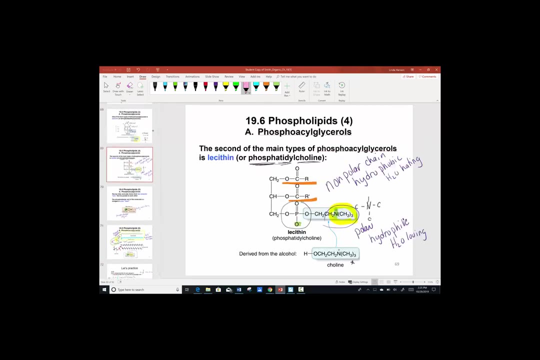 going to balance the nitrogen. that is all four bonds, NH3+. Now remember. Okay, So we have to remember cephalin, that cephalin molecule, just so we can see. I have to kind of go back up. Remember how we emphasized cephalin had just the three hydrogens attached to the nitrogen. 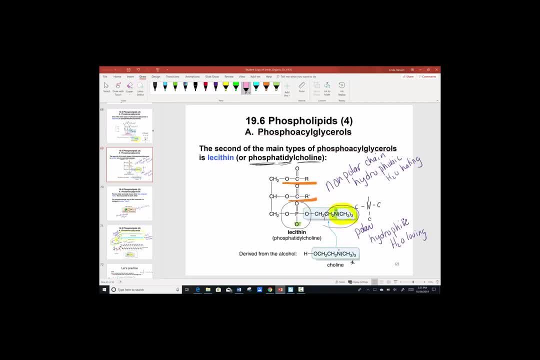 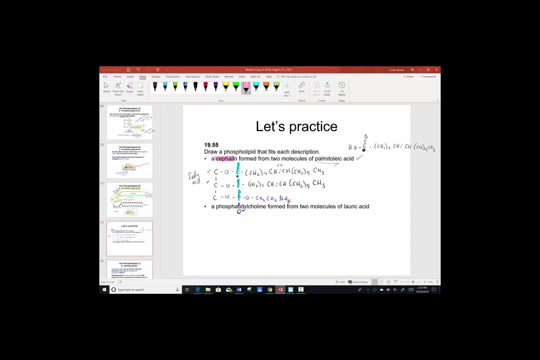 And to just emphasize the difference, on the next page we compared that to lecithin, which had all methyl groups around the nitrogen. Since this question asks us to draw a cephalin, We knew that it had nitrogens here at the terminal end to all hydrogens. 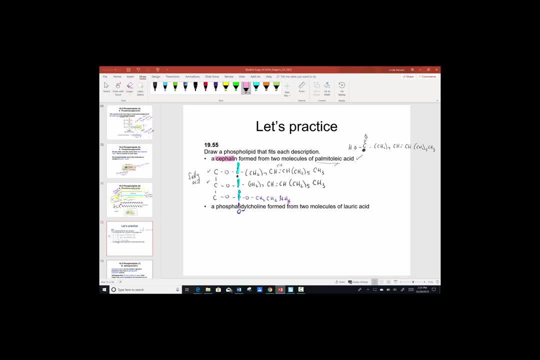 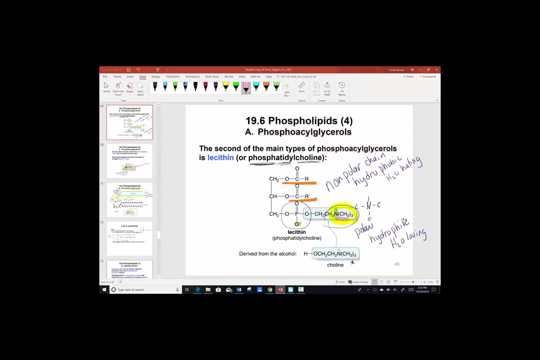 This next question asks us to draw a phosphatidycholine from two molecules of lauric acid. Well, where did we see that word a moment ago? That choline molecule, if you recall, was this particular molecule right here. how we 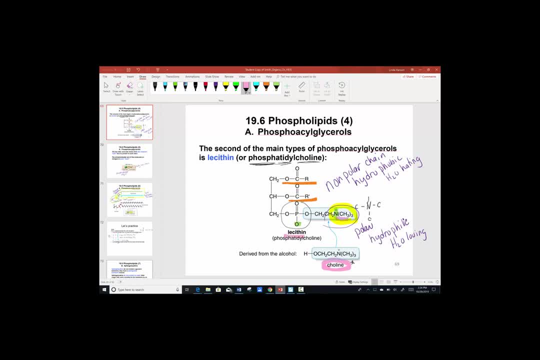 just emphasized a lecithin. A lecithin is coming from a choline and that's a tri-substituted methyl group on the nitrogen. So that's where I'm pulling this next example from, so we can see a model. 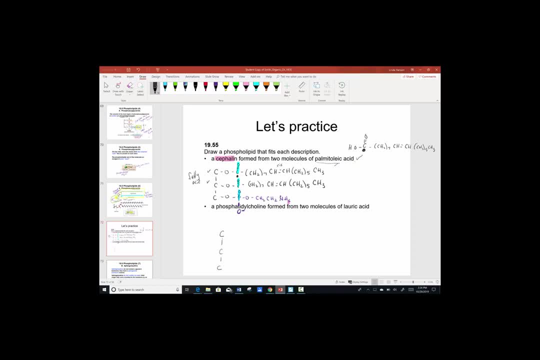 We always start with our glycerin backbone, CH3.. We will have ester linkages going in all directions. Now lauric acid. again, take a moment if you need to, because we have to look up. I don't know it by heart. 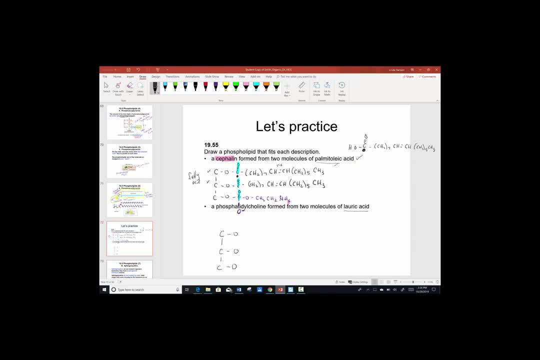 Maybe with enough repetition you could, But there's a chart on the front of your notepad for lauric acid And we can see that it is a carbonyl carbon. it's the acid. so we'll leave the OH there, even though when I come down to attach it it will form in an ester linkage. 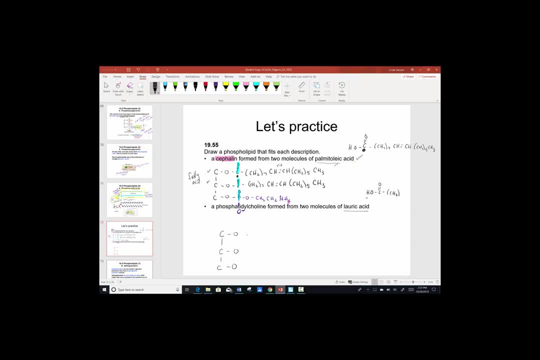 And this was a straight chain. So we had CH2 taken 10 times, leading to the terminal methyl group. So this is the lauric acid. How did you know that? Well, let's see. Well, it's in your table, on the front of your notepad page. 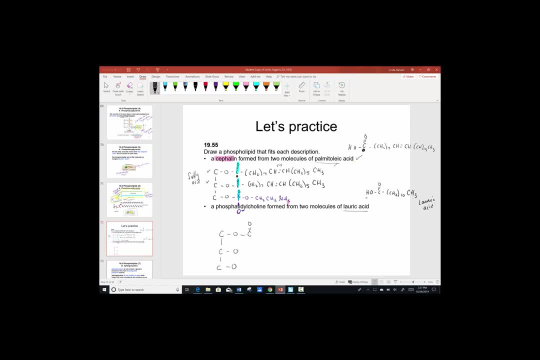 So that means right here I can just complete the two fatty acid tails by drawing in the carbonyl. That's this guy here. We had CH2 taken 10 times, terminating with the methyl group. That's a 12-carbon chain. 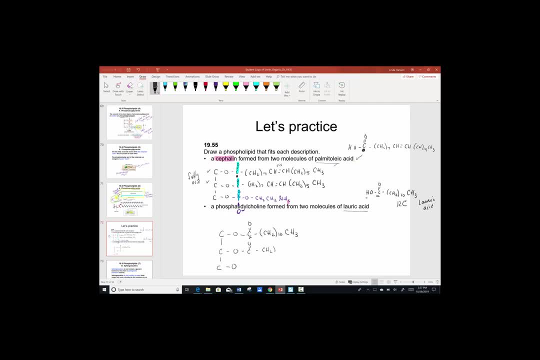 Position two will be identical, So I'll just repeat the second carbon, The two fatty acid tails, And that was the same as up here. These were called the tails, the nonpolar region that is hydrophobic, And this, of course, was known as the head of that molecule, the polar region of the molecule. 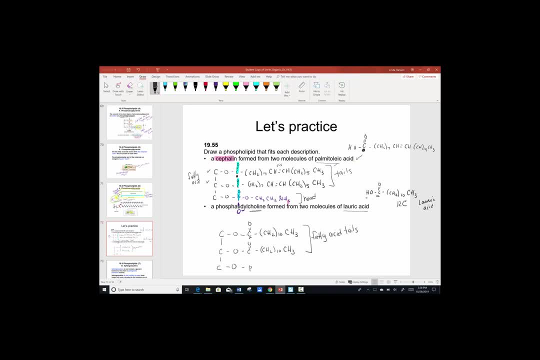 So now that we know we're coming from a choline, a phosphatidycholine, we're going to just follow that same example, But at the end we have all methyl groups attached to the nitrogen instead of. I'm going to make that O negative. 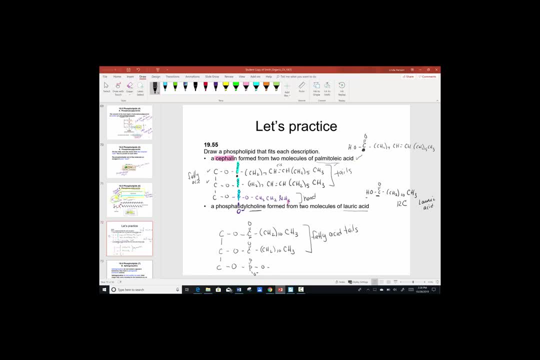 We lead to CH2 taken twice. I'll just jot them out: CH2,, CH2.. And now, at the end, the nitrogen has all methyl groups surrounding it in all directions. So it's N with a plus sign because it's four valent, four bonded. 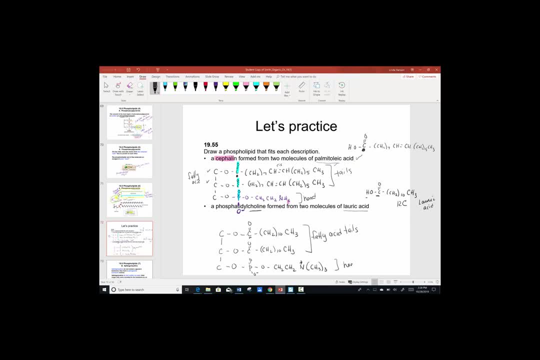 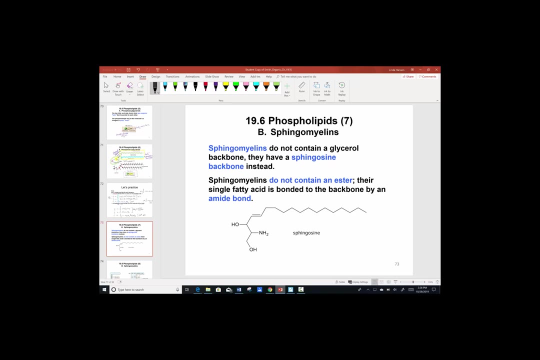 CH3, taken three times, And this is what we would refer to as the head or the polar region of the molecule We mentioned. there was a second category of phospholipids, a sphingomyelin. Sphingomyelins do not contain a glycerol backbone. 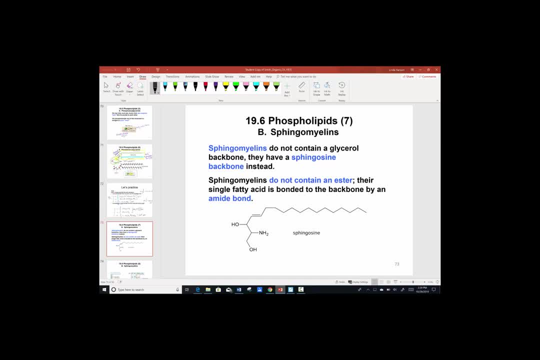 But instead their backbone is called phyngocine. Phyngocine, A phyngocine backbone instead. 1, 2,, 3,, 4,, 5,, 6,, 7,, 8,, 9,, 10,, 11,, 12,, 13,, 14,, 15,, 16,, 17, 18 carbons in the sphingocine. 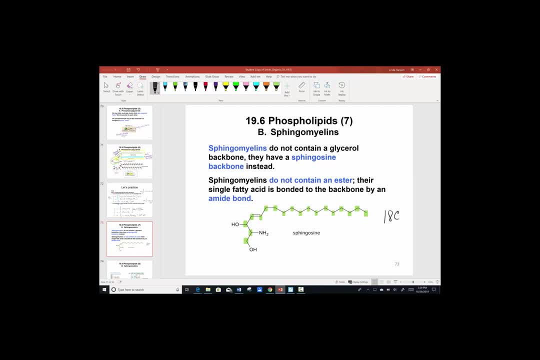 molecule sphingocine. That is the backbone, And notice the difference here In this section. this is a long carbon tail all by itself and does not need a fatty acid to create a second tail. So just part of the molecule itself really contains a fatty acid structure, doesn't it? 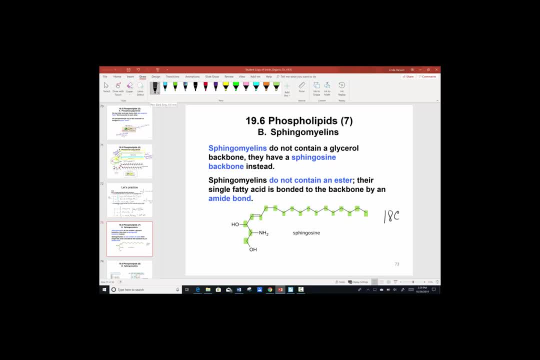 It's not truly a fatty acid because it never leads to an OH from a carbonyl, But it certainly is a nonpolar tail. That leaves a side of attachment then, Or two other functional groups. So when we think about that structural formula as a sphingocine that molecule itself gives 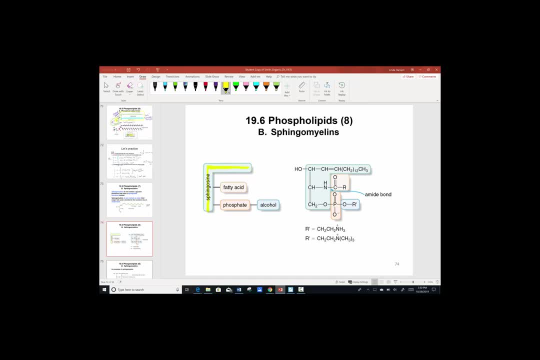 itself the first of the three tails all by itself. So here we have a molecule for a general structure, We had the fatty acid and then this was just like the previous: We have a phosphate attached to an alcohol, But the backbone is different. 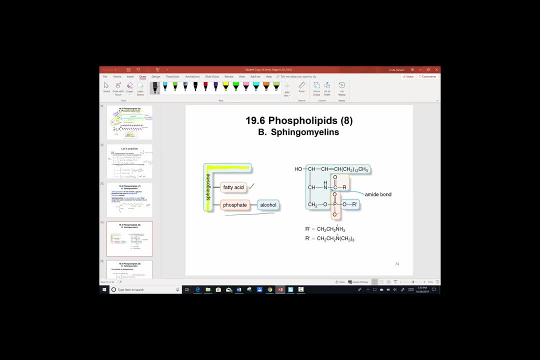 Instead of glycerol we have sphingocine. Now let's take a peek at some you know more focused. here We have carbon one, two, and at carbon two it leads to that nitrogen group. Let me back up and show you where that came from. 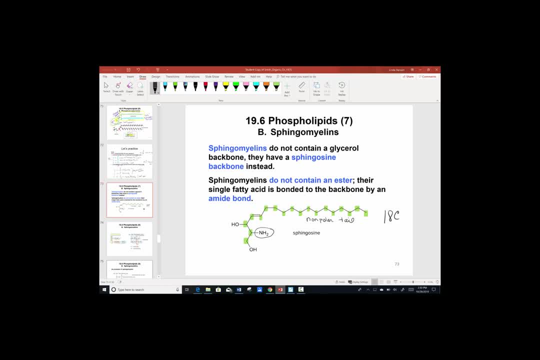 See this nitrogen group That actually is resulting in the next tail. So here that nitrogen group serves as a sort of attachment. This is what we called an amide. Again, the functional group. that's not right. the functional group where the carbonyl leads. 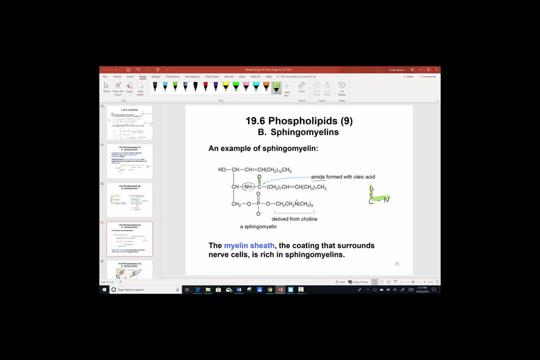 to a nitrogen. That's what's happening here. That's what's known as the amide functional group. And then of course we had the hydroxyl group, Remember. that's still sticking out here, So it's still kind of represented out here. the OH, and then the long carbon chain. that's 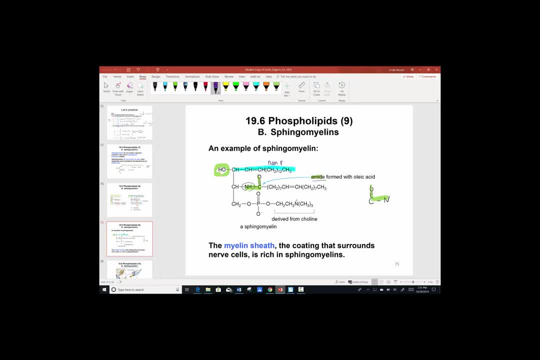 here, But it's still going to be a non-polar tail. So we still have a phosphodiester linkage. The carbon leads to an oxygen and instead of a carbonyl it now leads to the phosphorus. This is known really as the myelin sheath. 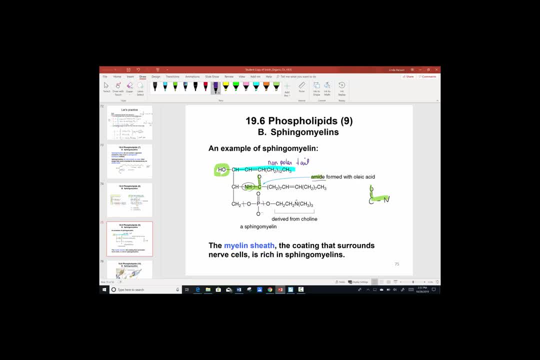 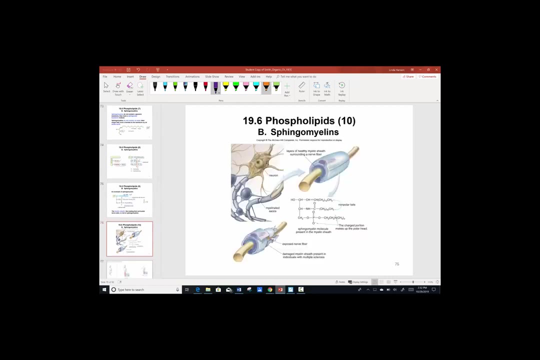 It's the coating that surrounds nerve cells And very rich in sphingomyelins. That's a coating on the nerve cell, help the axons conduct electrical current quite quickly down a long axon and dendrite. So if we just kind of take a peek, it's a basic cell here, a nerve cell from biology. 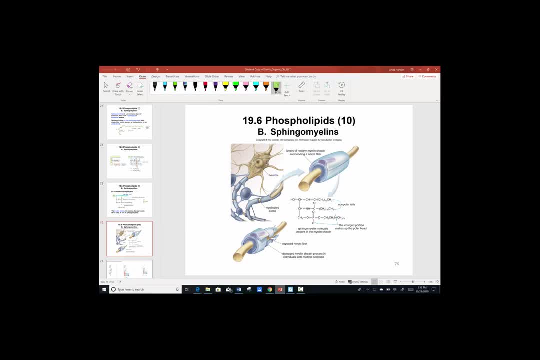 This is known as a neuron, and the neuron, of course, is responsible for creating electrical impulses that will stimulate an action. where the fiber ends, A myelin sheath surrounds the nerve cell and insulates that, and that insulation then says, as the electrical impulse originates from the nerve cell, it is allowed to just jump. 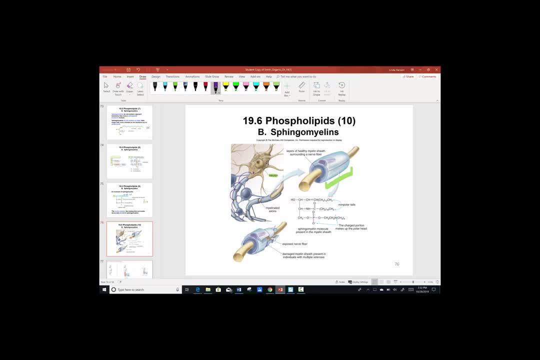 from axon to axon there And this coating here, which is a rich fat molecule kind of insulates interior and helps conduct a faster current by allowing it to jump from node to node. So again, here is an example Of a sphingomyelin molecule, the sphingo. this is the tail here, this is the whole backbone. 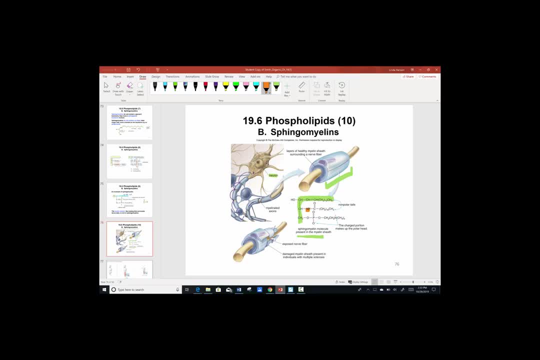 molecule here and notice that it contains a nitrogen group and the hydroxyl group is all part of the original backbone. the original backbone we called from the sphingomyelin, So that backbone itself. just trying to say some words here: sphingosine, sphingosine. 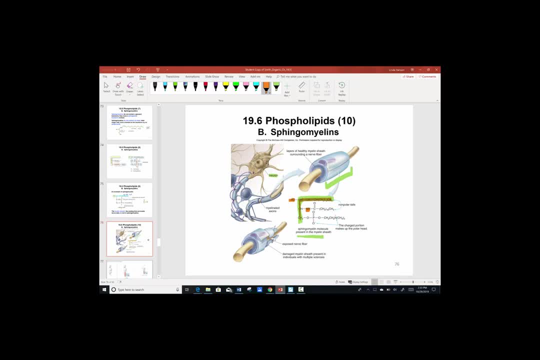 that's the sphingosine, This particular backbone. Part of that structure included an amino group and a hydroxyl group. We have the charged particles here of the oxide negative when the nitrogen positive just based on formal charge and long polar tails or long nonpolar tails as part of the 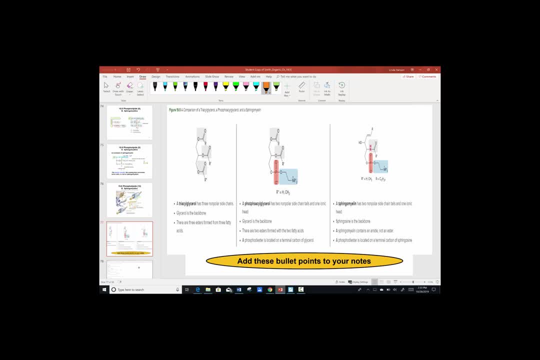 compound, And this makes a nice reference. you might even want to pause the video here and just add these bullet points to you. I want you to compare and contrast the picture of a triacylglycerol, the triacylglycerol that 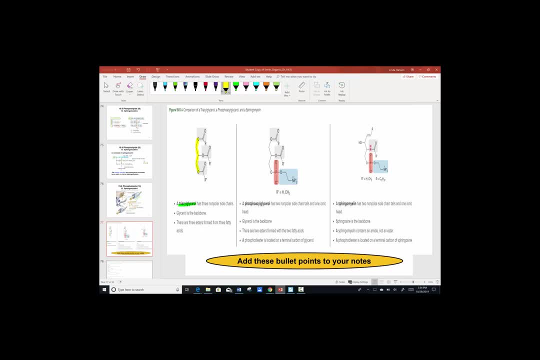 had the glycerol backbone, which is the three carbon unit, and all three of the attachments were just fatty acid chains: triacylglycerol: Three ester linkages leading to three fatty acids. You then compared that to phosphoacylglycerol. 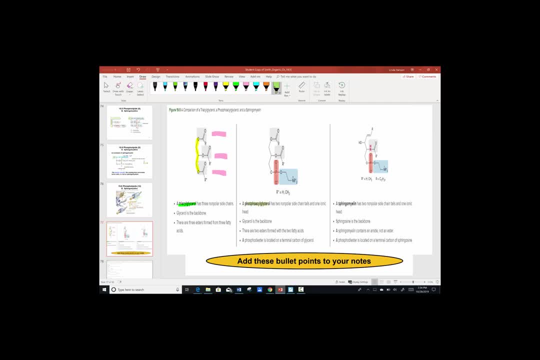 Phosphoacylglycerol Stem Still contained the same backbone: carbon 1,, 2,, 3, that's the glycerol backbone, And still identical is two of the three fatty acid chains. And what's unique is the phosphate linkage, the diester-phospho linkage, leading out to 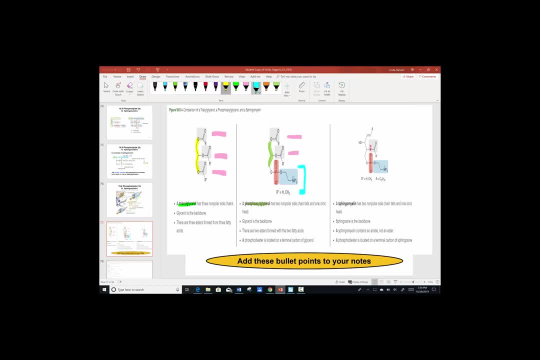 a nitrogen group. And then, finally, the third molecule had a completely different backbone: The sphingomolecule. The sphingomolecule has two nonpolar side chains and one ionic head, and that molecule is called sphingosine. 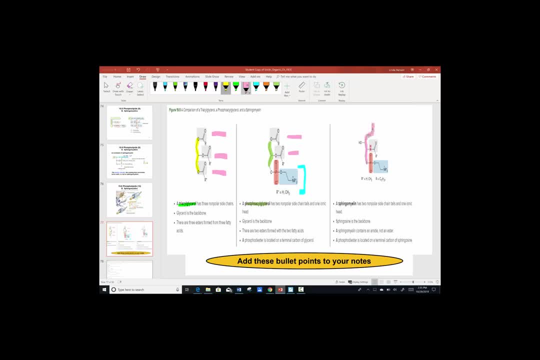 This molecule represents the backbone and we saw as part of it we had a hydroxyl group and the amine group. This part leads out identical. let's make sure we can see that I'll use bright yellow. These two are identical to these structures. it's the backbone that's different and this: 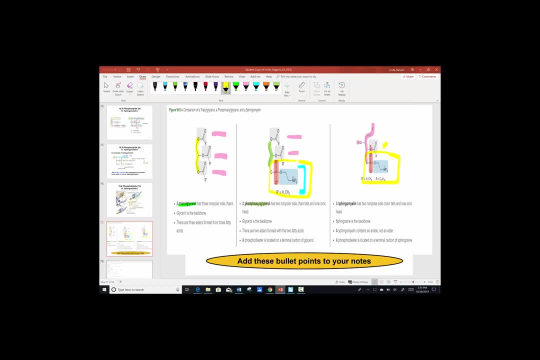 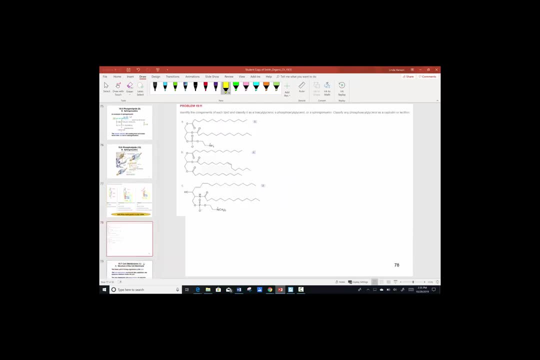 is different here from the nitrogen in position 2.. Add those bullets and it helps to emphasize the structures as we're working to memorize. Let's identify the components of each lipid and classify it as a triacylglycerol, a phosphoacylglycerol. 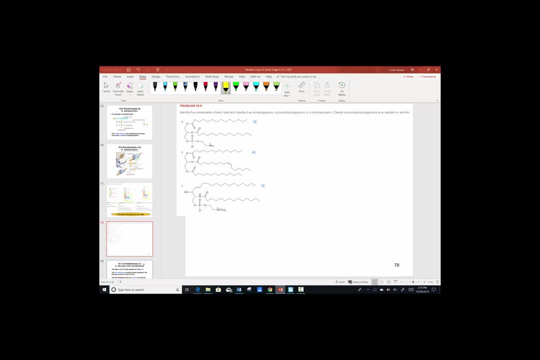 or as a sphingomyelin. Classify any phosphoacylglycerols as cephalin or glycerol, And that's it, Thank you. Thank you, Let's start on polyxythin, All right, So let's start by finding the backbone. 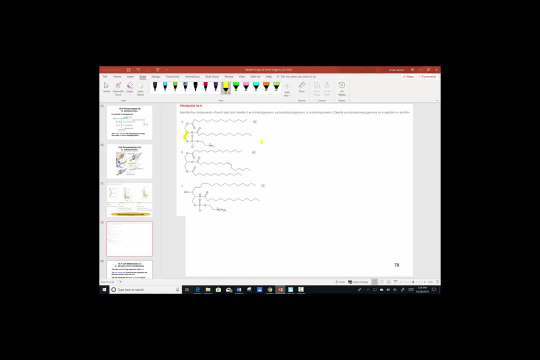 All right, so I have carbon 1,, carbon 2, carbon 3, leading to ester linkages. So this I recognize as a glycerol backbone. I then recognize the long carbon fatty acid chains, so I have two fatty acid chains. 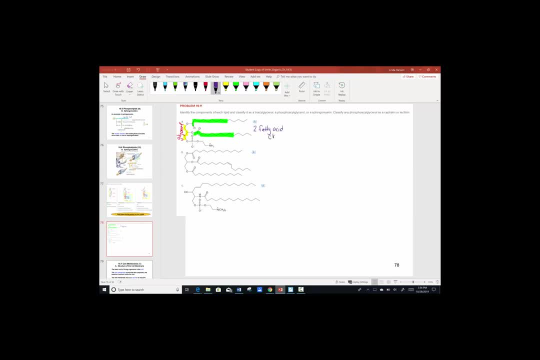 There we go. And now, if this last linkage were the same, I'd have a triglycerol, but they're not. I have going out here. I'm leading to a phosphate group And very critical is that the phosphate group has all hydrogens. 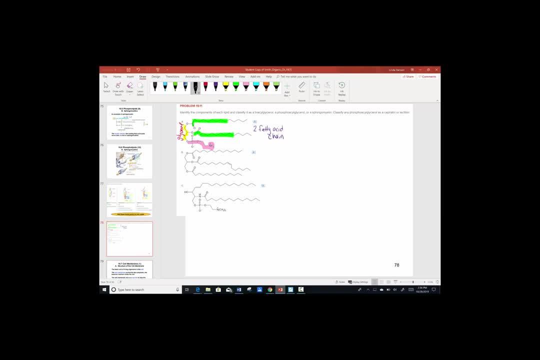 And when that's the case, we understand that it will now be categorized as a phosphoacylglycerol. And specifically, what type Is the cephalin? because they had all hydrogens leading out from the nitrogens. Let's peek at letter B. Letter B, I can recognize a glycerol backbone, a three-carbon chain. 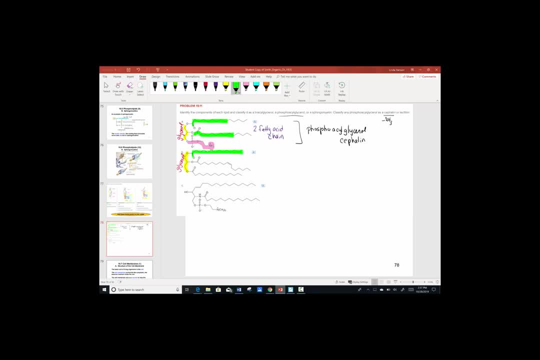 The first carbon chain comes all from fatty acid, The second is a fatty acid and the third is a fatty acid. All three are fatty acid chains And I know that because they're parents. The three fatty acids here are all carboxylic acids. 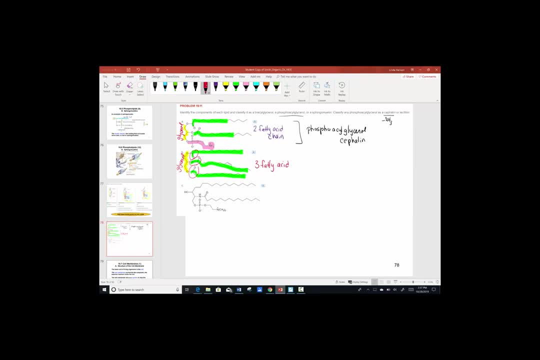 The word acid, carboxylic acid and the long carbon chain are fatty acids. So a glycerol with three fatty acids, we've learned is called a triacylglycerol. And how about this last one? We have something way different going on in the backbone. 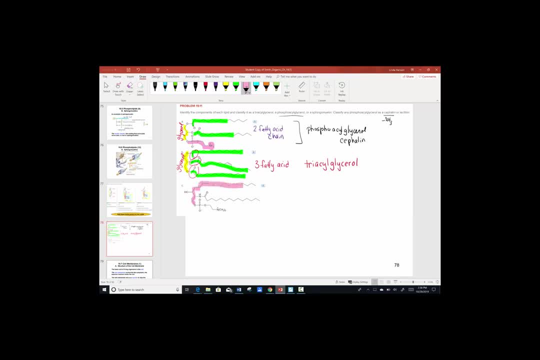 With the backbone. I notice, Okay, That I have a hydroxyl group off one end, I have a nitrogen group coming in the center And that, with this particular molecule, this whole entire structure serves as the backbone. I have a amine group coming off of position two. 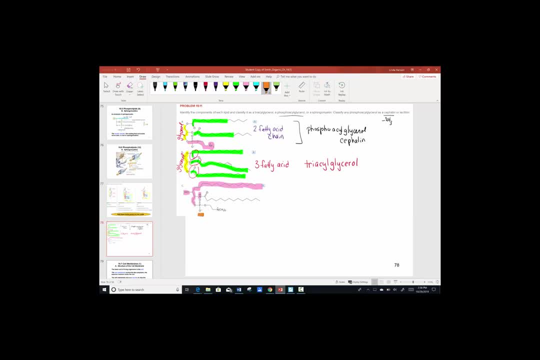 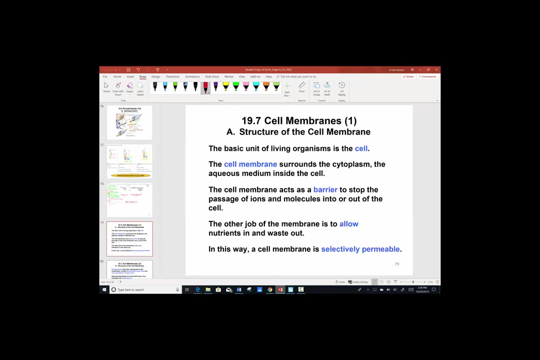 And I have a phosphate linkage coming off of carbon three. This is what we've learned to call a sphingomyelin. Okay, So this is what we've learned to call a phospholipid, And this leads to a very important application of phospholipid chemistry in any living organism. 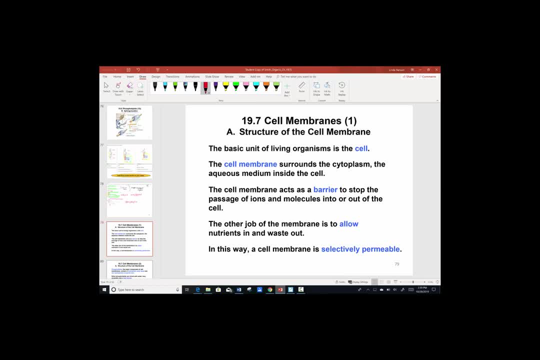 because it's the basic surrounding the membrane of a cell. We understand that the cell plays a vital role in creating an internal environment from the external environment and that cell membrane surrounds the cytoplasm. And I remember even in biology days of high school, oftentimes students would just be: 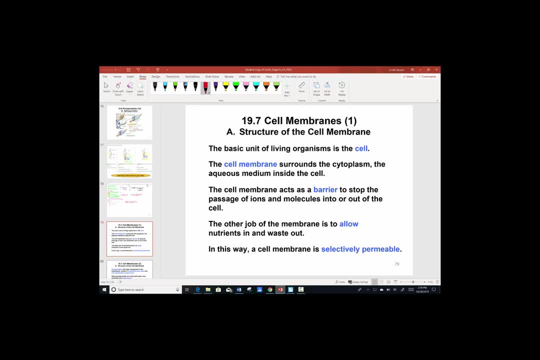 asked to draw a cell membrane or even a cell itself and make you know, label it out. So we're just reminding ourselves that a cell membrane has been called a phospholipid bilayer and it serves as a barrier to keep certain ions out and certain molecules in. 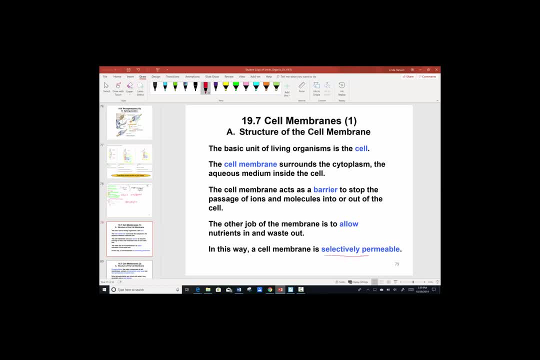 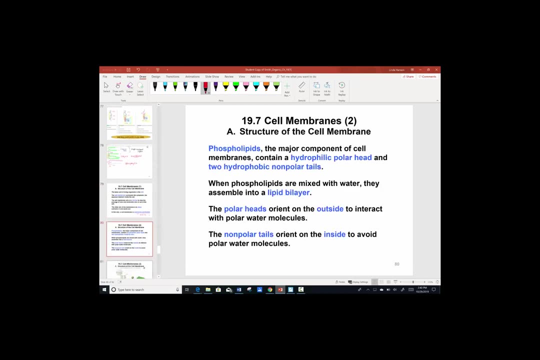 Semi-permeable. Okay, Semi-permeable. Sometimes we hear it called selectively permeable. It's the job of the membrane to allow nutrients in and wastes out selectively, based on the polarity of the substance. So those phospholipids with their hydrophilic polar head and two hydrophobic non-polar tails. 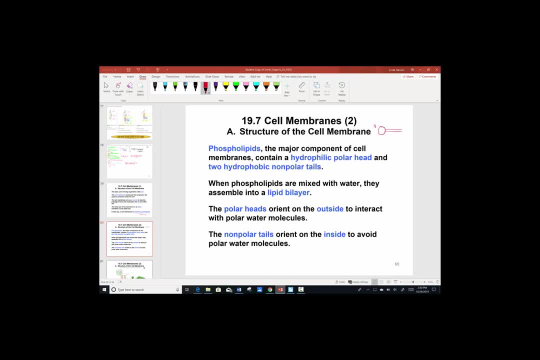 that's this general structure we saw before. We had the head, Which is water-loving, And we had the tail, which is water-hating, a phospholipid, And we call it a bilayer, because we can start layering these one on top of the other to 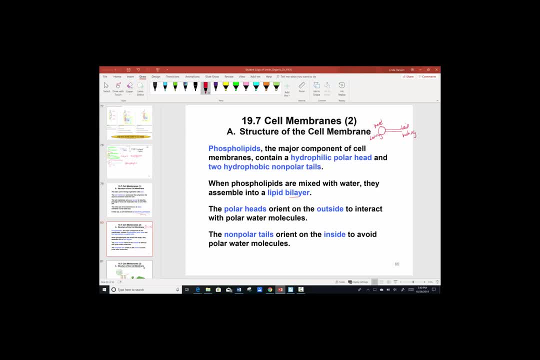 keep the polar heads on the outside. So, as I draw this structure, if the polar heads are facing to the outside environment, what it will do is be allowed to interact with the water on the external part of the cell, Simply because these are polar or water-loving and therefore they have an interaction that's favorable. 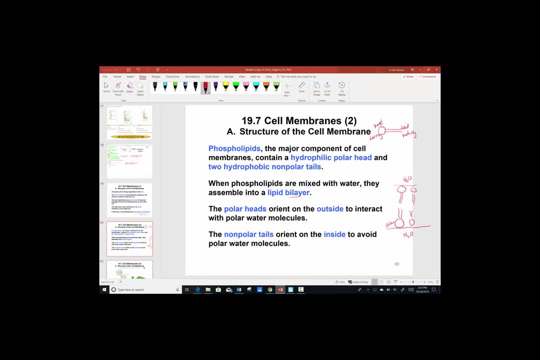 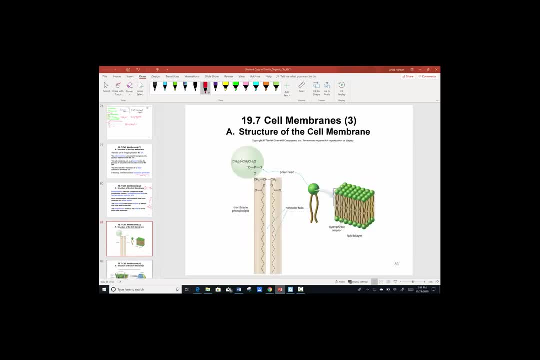 The non-polar tails are to the inside to avoid because they hate water. right, The non-polar tails avoid the water by pointing inside. And here's a structure far better than the one that I just drew. Here is the head, the phosphate ion. 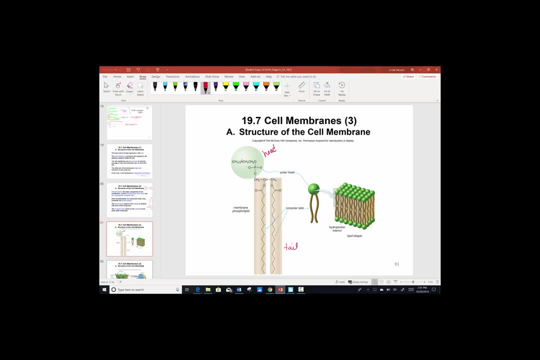 Here is the tail, Those long carbon fatty acid chains and that general structure, the heads and the tails, And we call this a phospholipid bilayer, where the heads point out and the tails point in: Hydrophilic, hydrophobic. 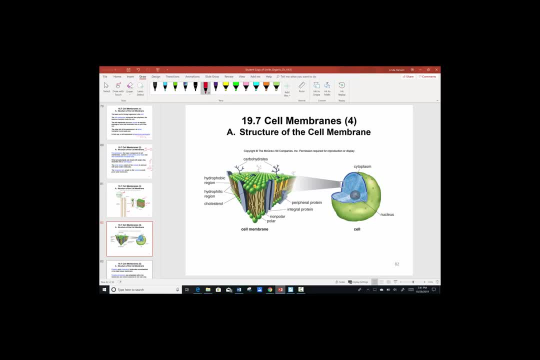 0, 0, 1, 2, 3, 4, 5, 6, 7, 8, 9, embedded in the cell membranes to ease transport across the cell membrane. Some of the things you see might be a carbohydrate. You might see an integral protein. 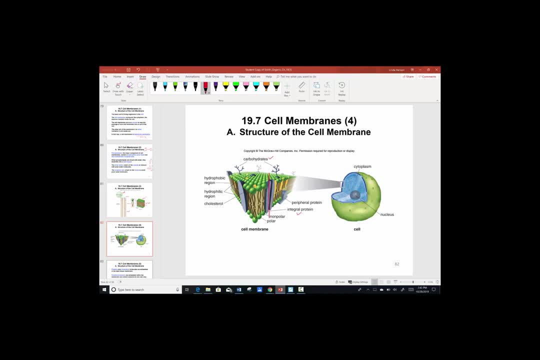 An integral protein goes all the way through the entire membrane, Or a peripheral protein which just is embedded at the surface. You could see a cholesterol molecule embedded in there to give it rigidity And you see hydrophobic tails, hydrophilic heads, all part of a cell membrane the selectively 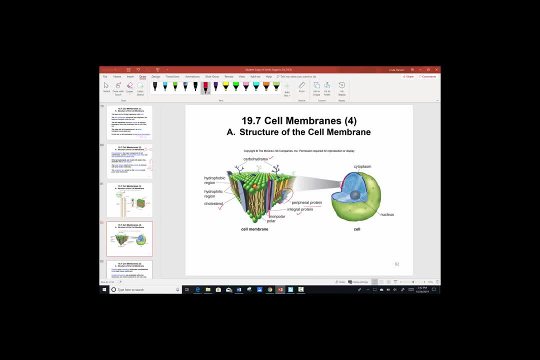 permeable membrane that allows certain substances in while keeping others out. Those proteins and cholesterol molecules. well, they're embedded in that phospholipid bilayer membrane. as pointed out, We said that peripheral proteins were embedded just on one side. Integral proteins extend the entire way through. 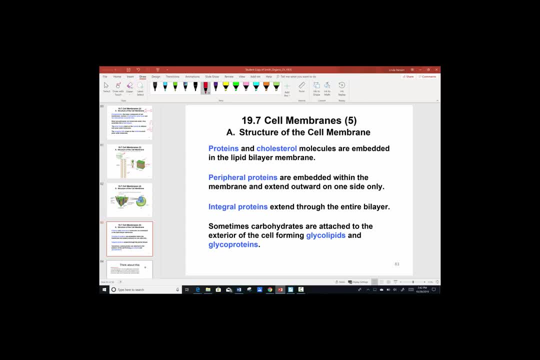 The phospholipid bilayer, And sometimes you'll even find carbohydrates that are attached to the exterior of the cell, glycolipids and glycoproteins. Upcoming chapters, of course, will talk further about carbohydrates and proteins and amino. 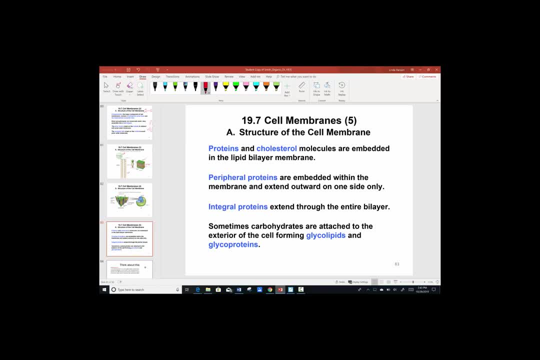 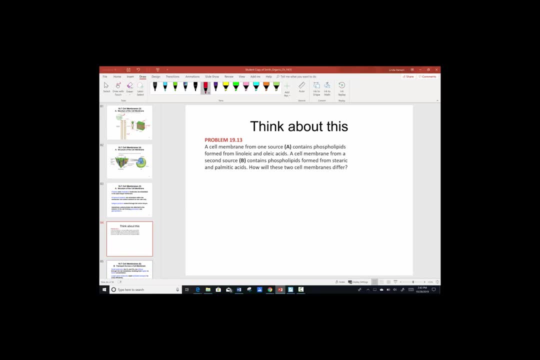 acids and so forth. So we're just saying the words to help ease into that next topic on proteins. A cell membrane from one source contains phospholipids formed from lenaic acid and oleic acid. A cell membrane from a second source contains phospholipids from stearic acid and palmitic acid. How do 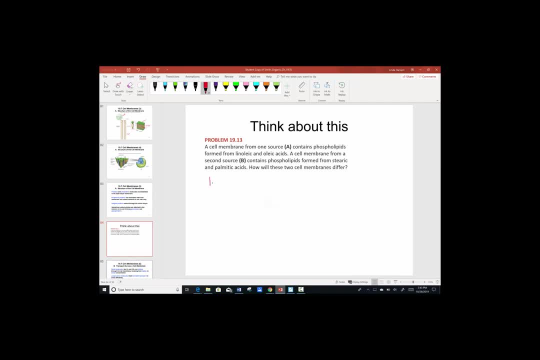 these two cell membranes differ. Pull out your chart with the very front cover and find for me the formulas for lenoleic and oleic acids. Let's do the same from stearic and palmitic. I want you to decide which ones are saturated and which ones are unsaturated. 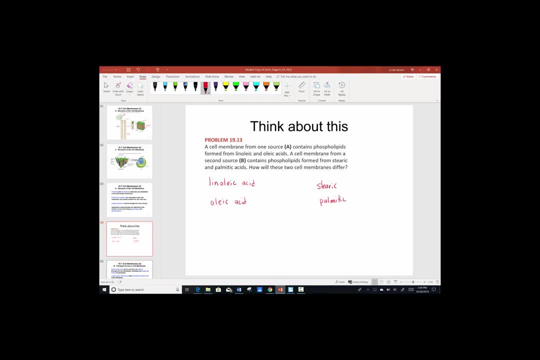 as you kind of tackle that problem. I don't want to just give the answer without some think time, But I'm hopeful that you'll find the answer as you think deeper into what type of structures you're looking at. What do lenoleic and oleic acid have in common? What do stearic and palmitic? 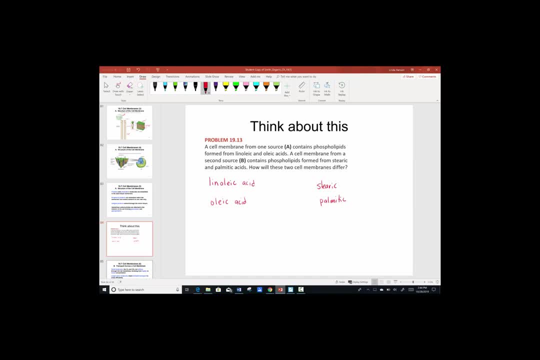 acids have in common, And I'll pull out my fatty acid chart and we'll kind of look at that together. See if I can find one. Did you find yours? yet Mine is not closed, are it? Well, hop, Eureka, Maybe I beat you, maybe you beat me, I see. 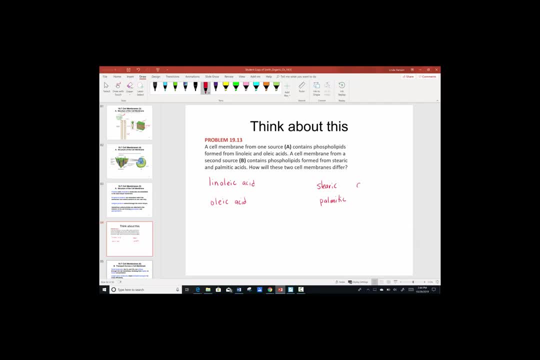 that stearic acid here is CH3, CH2, and that's taken six times. COOH, And that's taken six times. And palmitic acid is the one right above it. This is CH3, CH2, taken 14, I think. 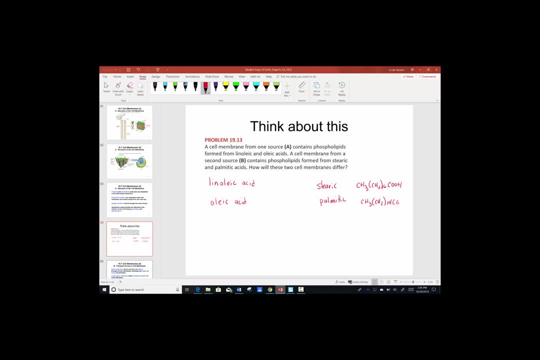 that's a 16,, my bad 14, and that's COOH, But I wanted us to notice that these are saturated fatty acids. That's the key in recognizing their commonality is that these are all single bonds, And what similarity did you notice with lenoleic acid? 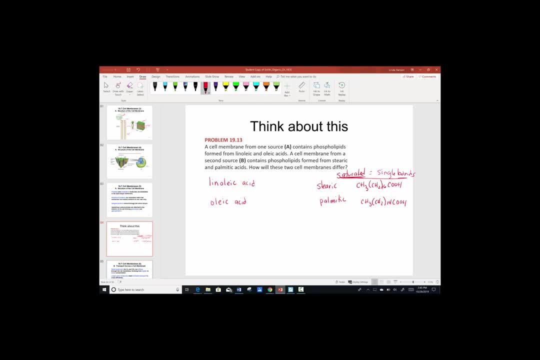 Oleic acid and oleic acid, Well, lenoleic acid. as we look on this chart, this had CH3, CH2, taken four times CH, and then we start to see some double bonds And there's quite a few double bonds, And I'm just going to quit writing there, because we just recognized 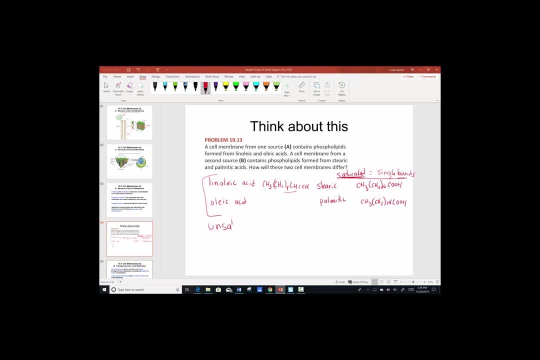 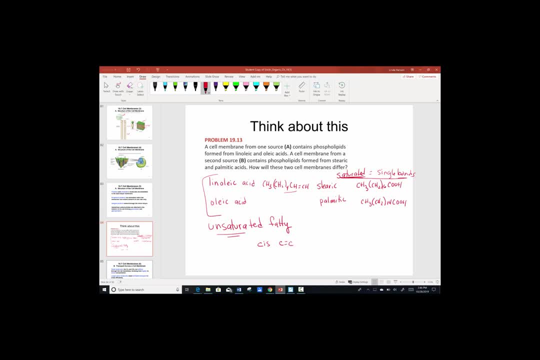 with those cis-double bonds make them liquids at room temperature, and saturated fats are solids at room temperature. So, as I interpret this question, it's really asking me: what difference does it mean if the phospholipids are liquids at room temperature or if they're? 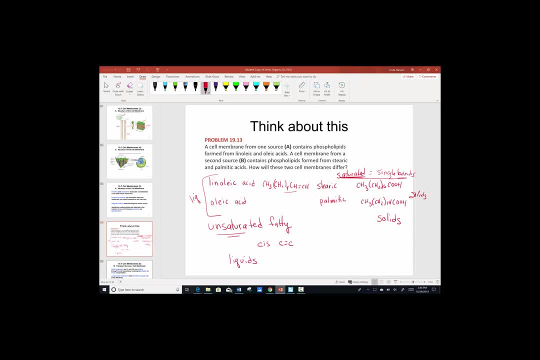 solids acids at room temperature. how might these two cell membranes differ? And that kind of eased into the answer a little bit, didn't it? So I would expect membrane A, with these unsaturated fatty acids, to be more liquid, more fluid. 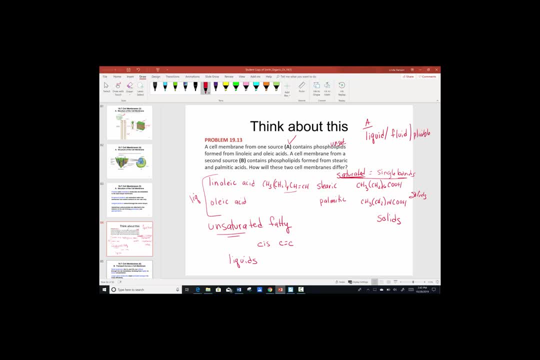 more pliable might be another good word, Since they are contained with fatty acids that are unsaturated, whereas compound cell B, which their fatty acids are saturated, coming from very tightly packed, more rigid. The rigid part I'm just kind of emphasizing because we know that it would come from a 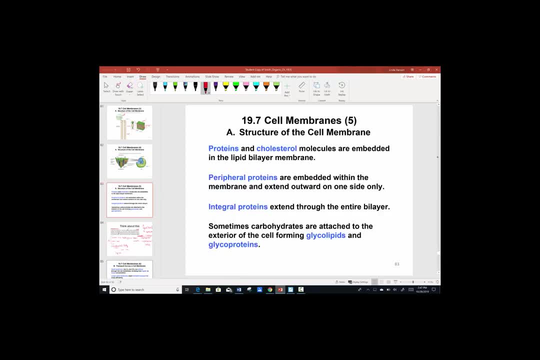 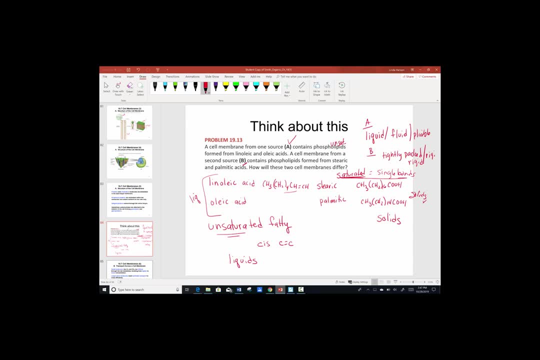 solid instead, so more rigid. I think I ran out of room. that's why it keeps jumping there. All right, All right, rigid underneath. So, in the presence of our unsaturated fatty acids, we have a very fluid, a very liquid. 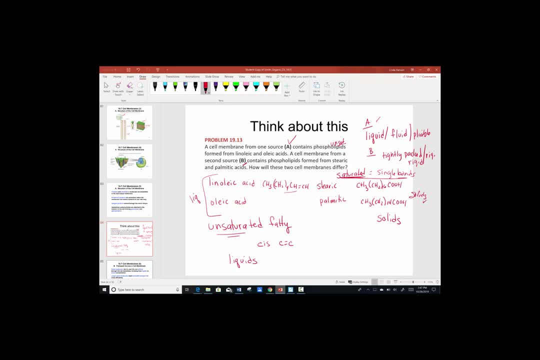 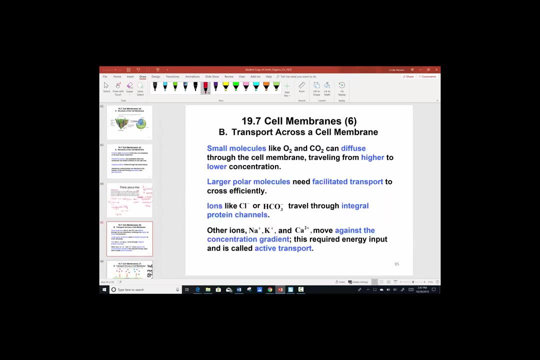 and pliable cell membrane, whereas if the cell membrane is made of phospholipids with fatty acids that are saturated, it's a much more compact, more tightly produced packing and then rigidity, And that makes sense just based on the structure of the fatty acids contained in there. 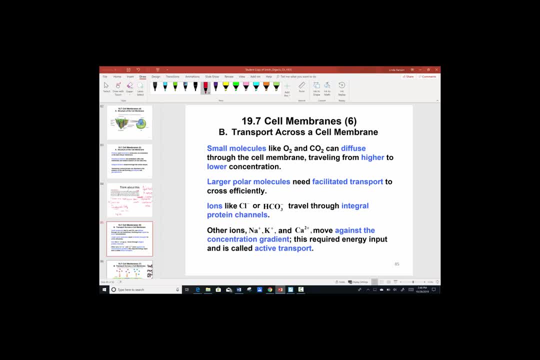 And of course we know that transports across The cell, and this is again a little review from your biologies. these small molecules can diffuse right through based on what we call diffusion. Diffusion is defined as motion of a molecule from higher to lower concentration. so just 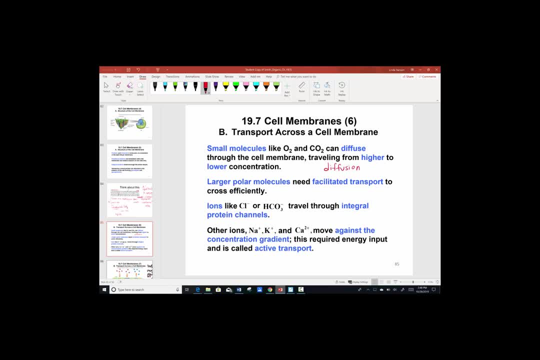 based on a concentration gradient. The larger polar molecules need to be facilitated to transport and that's the job of that facilitated protein active transport. Ions can travel through the integral protein channels based on charges and some of them have to move against the energy gradient you know, from low to high concentration. 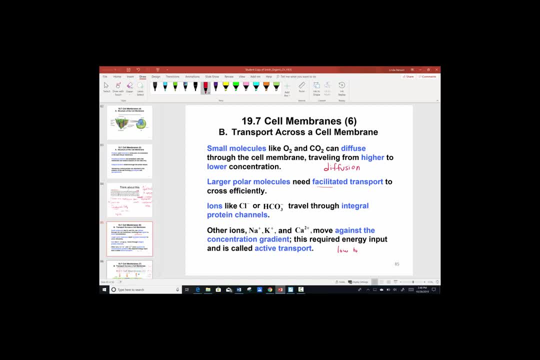 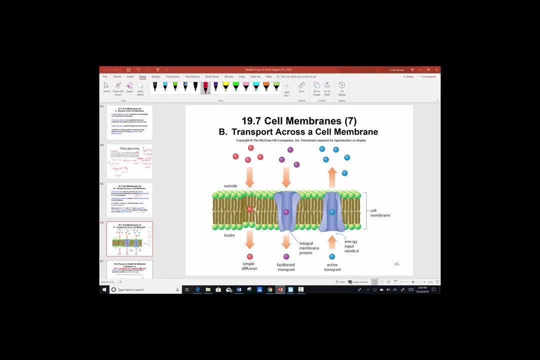 and that's not the natural state of diffusion. So from low to high must cost the cell energy to do that and that's why it's known as active transport, And I think a nice visual of all of those vocabulary words is simply placed right here. 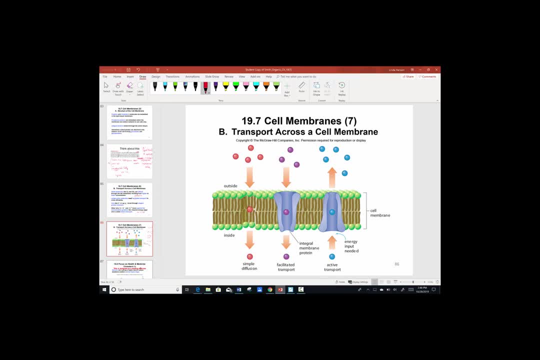 The cell membrane. if it diffuses directly through simple diffusion based on a concentration gradient. If it's allowed to go through a transport channel based on the gradient, we called it facilitated transport. If it's being pumped out of the cell against the concentration gradient, it costs the cell. 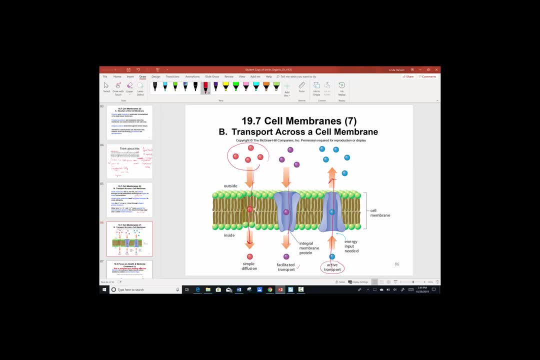 energy and will be called active transport, And that's why we see the energy being input. Recognize the phospholipid bilayer, the heads pointing out and the tails pointing in Great work with our talk today about phospholipids. 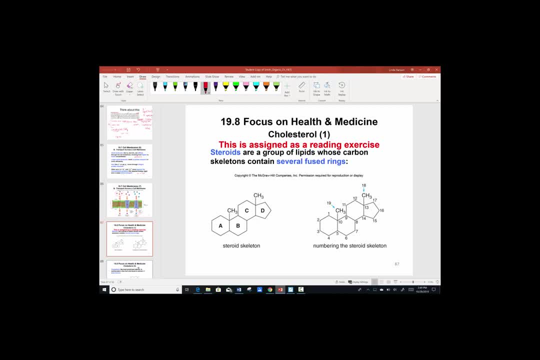 The rest of your chapter is now assigned as a reading exercise In your Section 8,. if you'll allow me to just preview Section 8, you're going to focus on health and medicine, specifically the cholesterol molecule. Okay, You'll see that steroids are a group of lipids whose carbon skeletons have several fused. 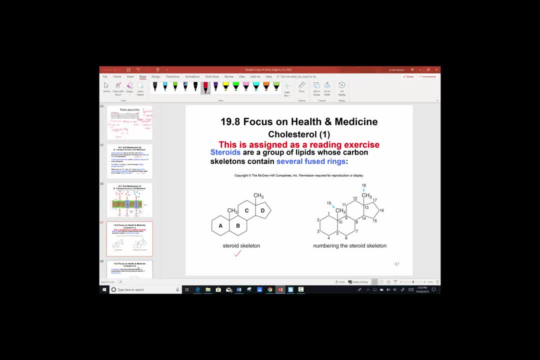 rings and you'll be asked to draw out the steroid skeleton and you'll be asked to number the skeleton. Now it is fine with me if you draw this once and just number the same structure. That's fine. I give you two boxes. 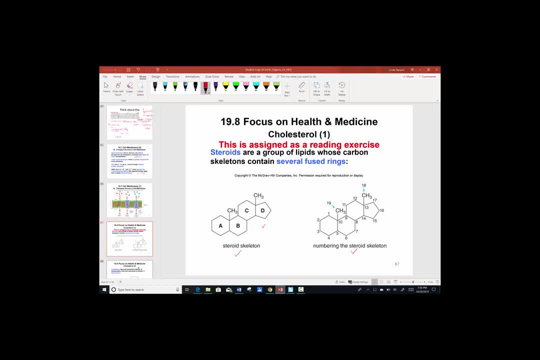 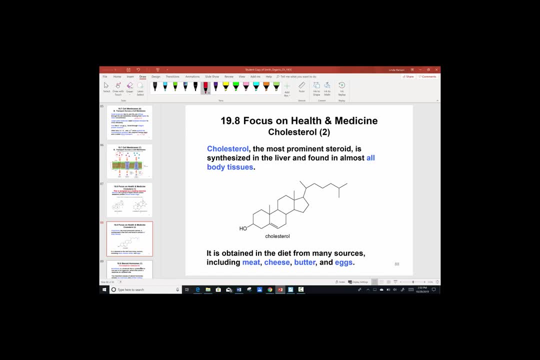 You decide, But you'll investigate steroids and their fused rings. You'll then turn your attention to cholesterol, which is the most prominent steroid. We talked a little bit about cholesterol and cardiovascular health in a previous lesson. Synthesized in the liver and it's found in almost all body tissues and we get that. 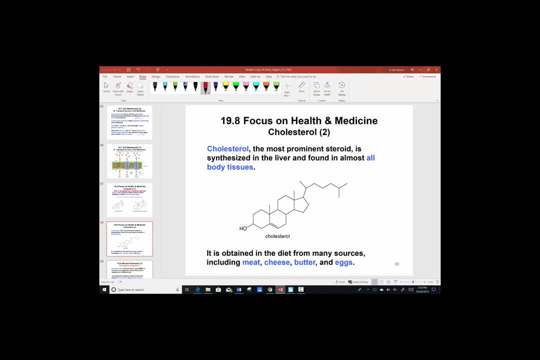 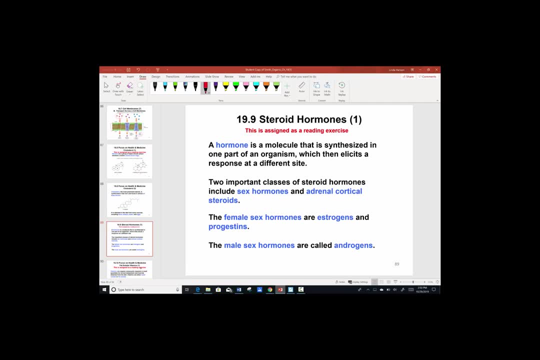 from many dietary sources, mostly from animal products: meat, cheese, butter, eggs, not so much in the plant. And then in your ninth reading section, your Section 9 is on steroid hormones, and you'll go through You kind of compare what a hormone is as a molecule that's synthesized in one part. 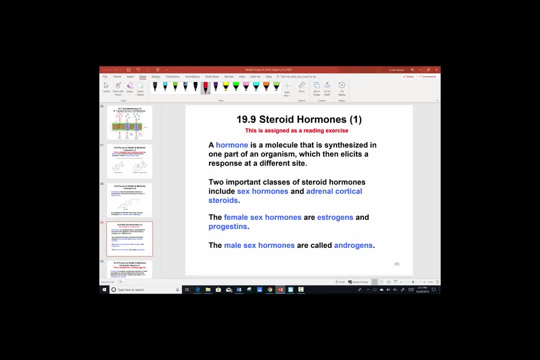 of the organism, but it doesn't have an effect in the immediate area. It actually elicits a response at a different site. So a hormone is a traveling messenger. You'll look at the chemical compositions of a few hormones, such as the sex hormones and. 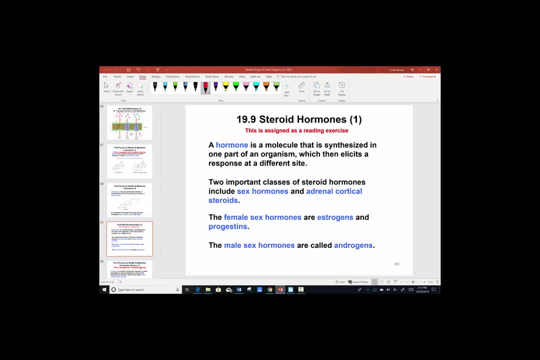 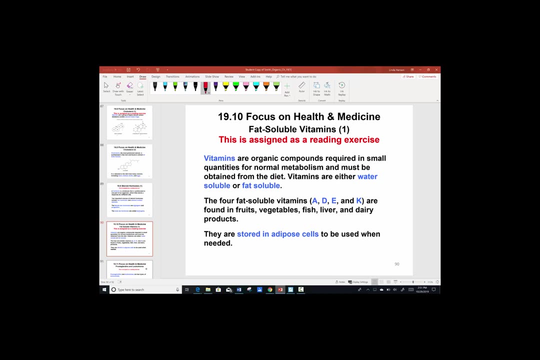 adrenal cortical steroids as well, and you'll look at the sex hormones of estrogen and progesterone and females and androgens in the male and you'll fill in that reading packet. You'll focus on fat-soluble vitamins and learn that vitamins are organic compounds. 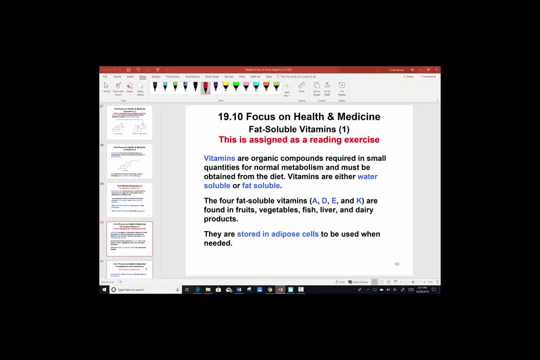 They come in two categories- water-soluble or fat-soluble- and we'll need to have those recorded as the fat-soluble so they're stored in your adipose tissue and not just flushed out. Any excess amount gets stored, unlike water-soluble vitamins. 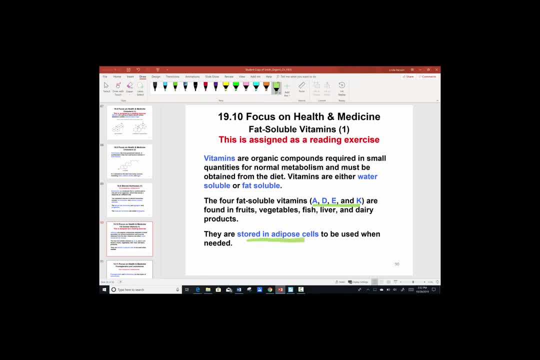 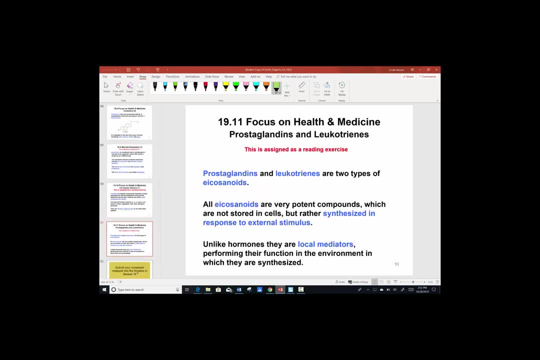 Just flush out any extra amount, So you'll read about how they store in fat cells and complete that section of your reading guide. And then, finally, the last focus on health, we'll look at prostaglandins and leukotrienes. 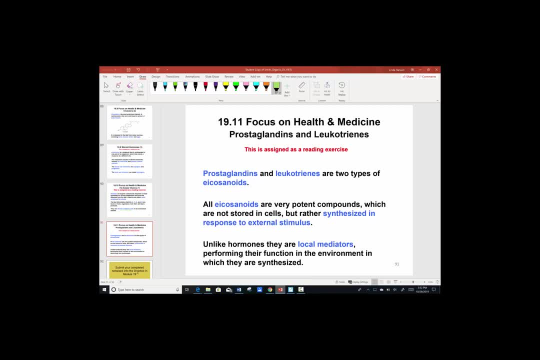 Leukotrienes and prostaglandins trying to say those words so you can hear them in your head. Prostaglandins and leukotrienes. you can hear the three double bonds of that word. triene. They're two types of this chemical family called eicosanoids, and read a little bit. 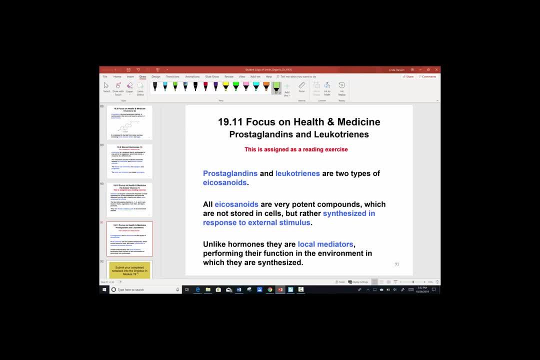 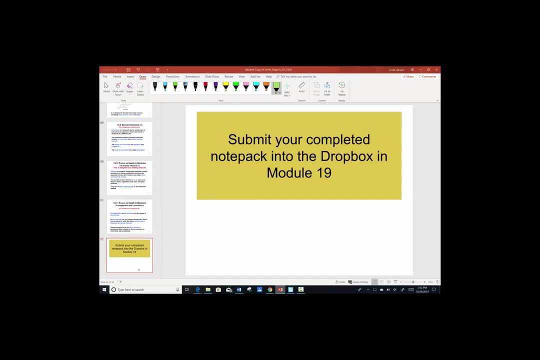 about how they're synthesized and how they're called: local mediators And friends. when your entire packet is completed, you will submit your completed note pack into the drop box in this module 19.. I look forward to receiving your work soon.